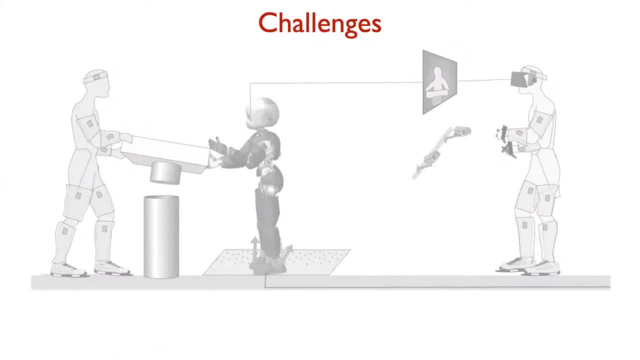 So what are The challenges when we do humanoid teleoperations? So there are many, but I will focus on three, maybe. So first, we need a generic whole body controller. Usually, when you see demos of humanoid robots, you see something that is autonomous, or sometimes teleoperated or commanded. 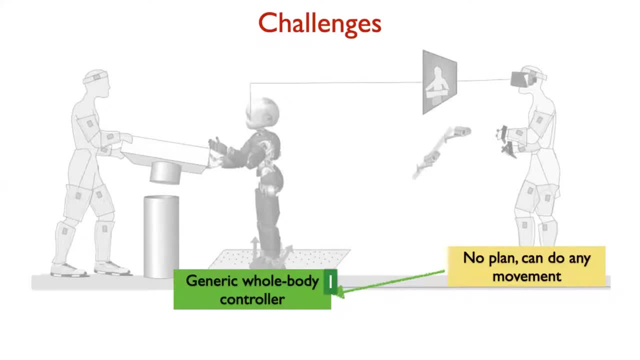 but in our case, the robot has to be capable of doing anything that the human wants, and the human is really commanding the robot to do, you know, whatever he wants. so we need a generic controller that is capable of doing whole body motions that are very diverse. second, the controller has to be: 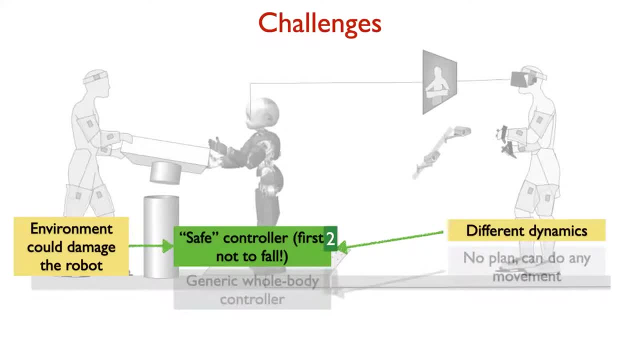 safe. i quote. so nothing safe in terms of proofs of safety, but first in the state, in the sense that the robot is remote on a remote location. first, it doesn't have to fall, which is primary concern. if the robot is damaged, he has to be able to continue the mission in its own way. and then 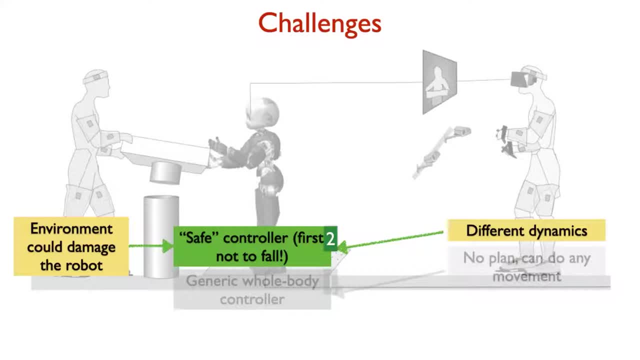 because of the targeting problem. so the difference between the dynamics of the operator and the human and the robot we need to take into account to prevent the robot to execute behaviors that are actually dangerous for a first movement. and then last problem is the delay. so when you are a human or a human that is operating a robot, even the smallest delays is a perturbation. 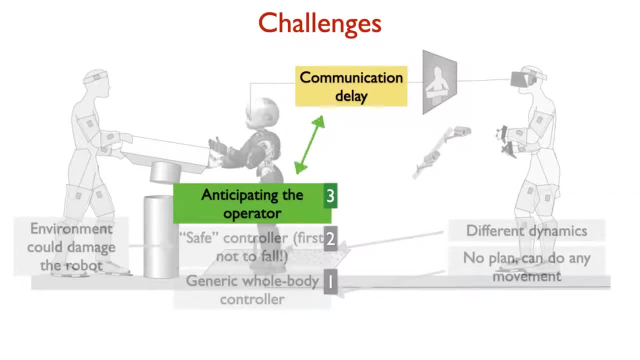 for you. so in some missions you have very long delays- that can be up to many seconds- and this is because it's big problems, so we have to find a way to compensate for these delays. so i'm gonna focus on, like, the three solution that we have on this problem. i'm gonna not gonna talk. 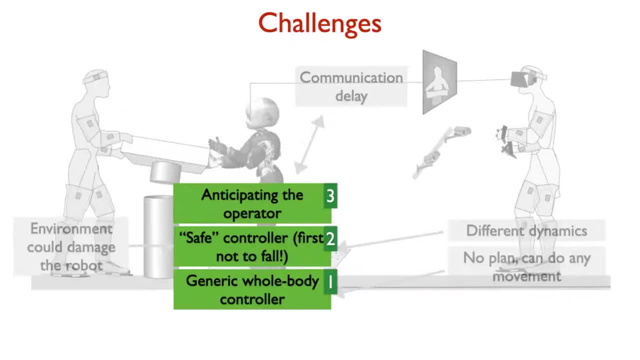 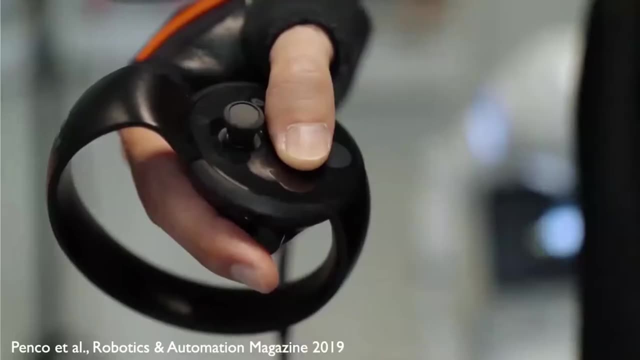 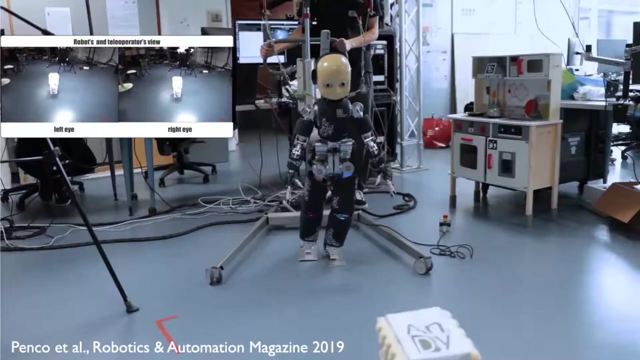 about the hri problem. like the operator interface. this is for other talks. so this is the uh interface. we had so since a couple of years now. so we are using an extent suit to target the entire posture of the human and we have a yes headset. so, uh, we are not. i'm not addressing working with the very 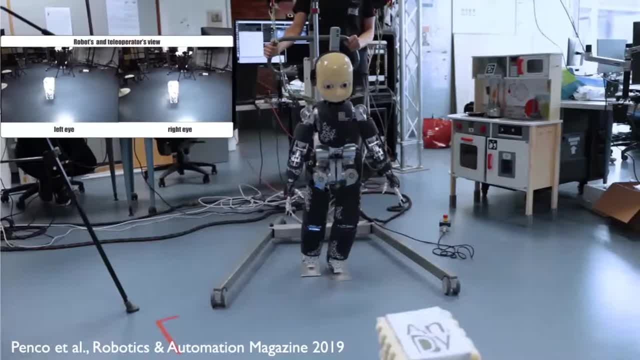 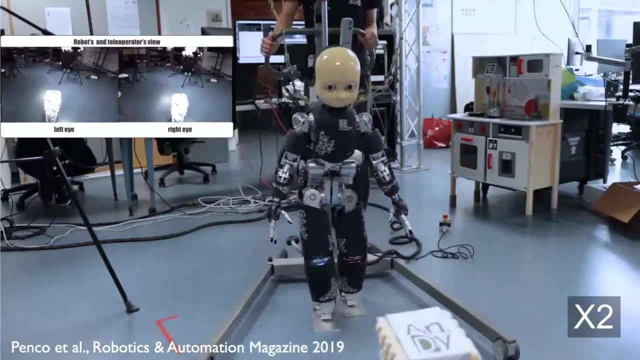 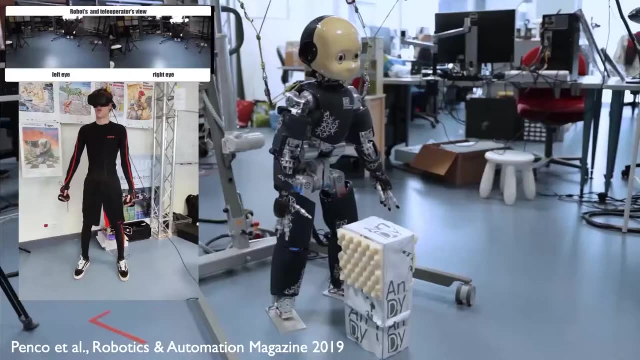 basic working that we have with the npc on the com and very simple world body controller, and the nice thing is that it's quite human-like at the end. so it's uh, yeah, it works. it's not very fast, but for- and the nice feature is, when we are uh commanding human, um, whole body motions, like in this case the. 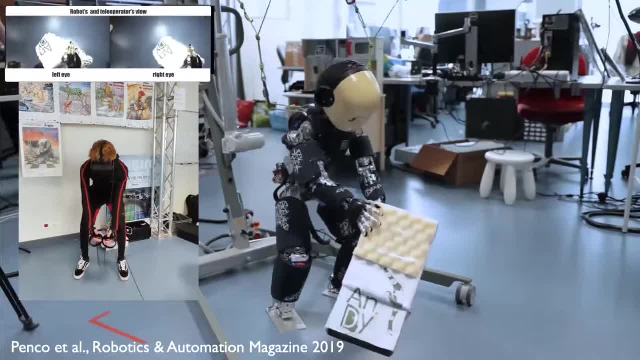 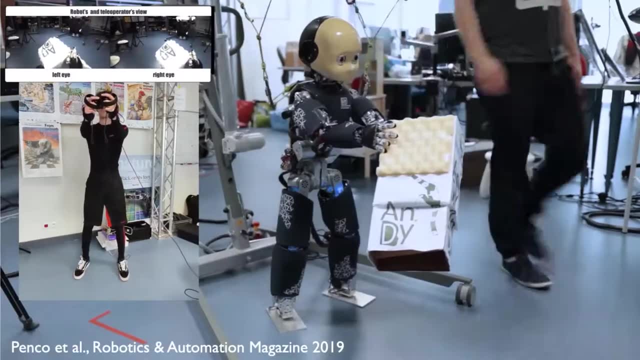 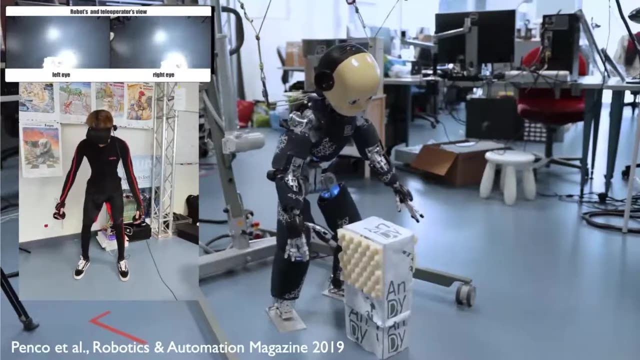 human is speaking something from the floor and then this is how basically it works. so, as you can see on the top, this is the view of the of the cameras. so the human is basically in the diagram that is looking at what the human human is, is seeing, which causes problems, and you will. 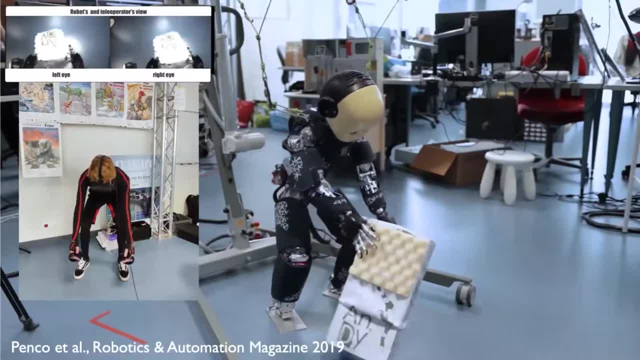 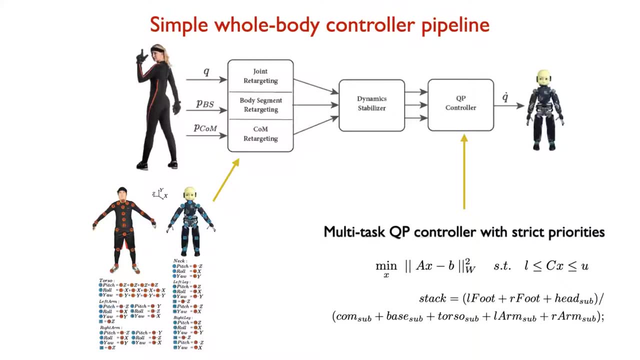 see later that we have another uh solution for uh give you more uh sort of awareness to the operator. so how does this work? it's very simple. we have a simple body controller pipeline. so we have a targeting part, some dynamic stabilization- that will come up later- and then our basic module is the world body controller. very simple with body controller. 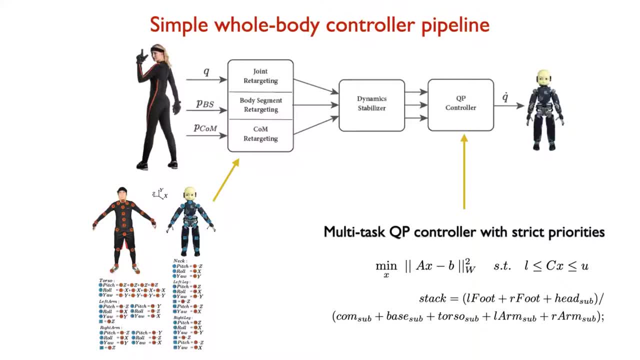 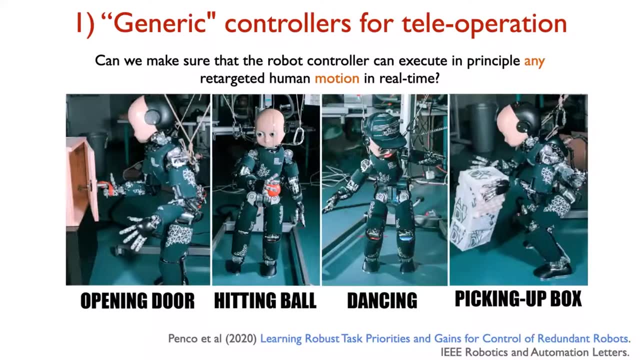 based on in the case of icab is what based on? it is based on stack of tasks, so it's mixing many different tasks with the strict priorities. so how do we make this controller that simple but plenty of? it has plenty of parameters, generic enough to be able to do many tasks and 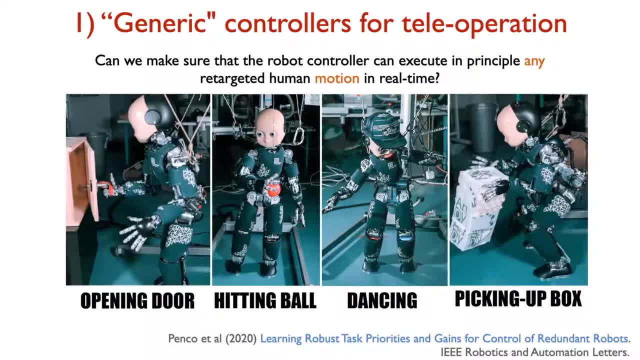 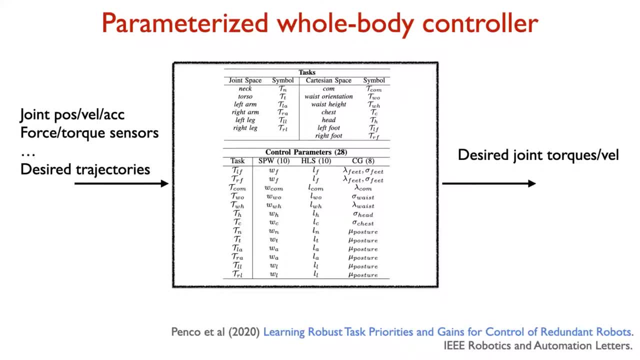 tasks could be opening doors, dancing, picking up boxes from the ground, whatever. so we turn this into a problem of parameters optimization. so at the end, the entire controller pipeline is just a box with plenty of parameters that need to be optimized. in the past, one engineer was tuning 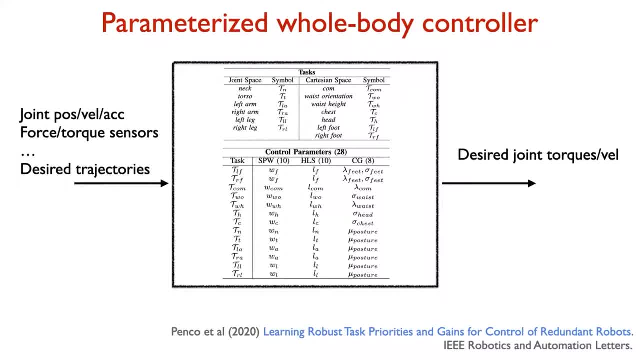 these parameters to achieve a very nice behavior. the problem is that if you achieve the parameters for picking boxes from the ground, you have a set of parameters that are not the same as picking something from the shelf or dancing when you want to be, track more the posture of the you want to be. 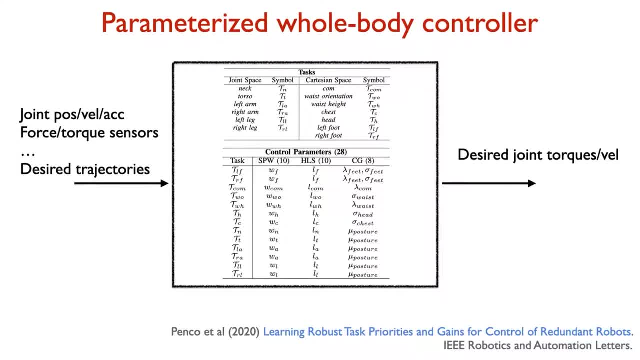 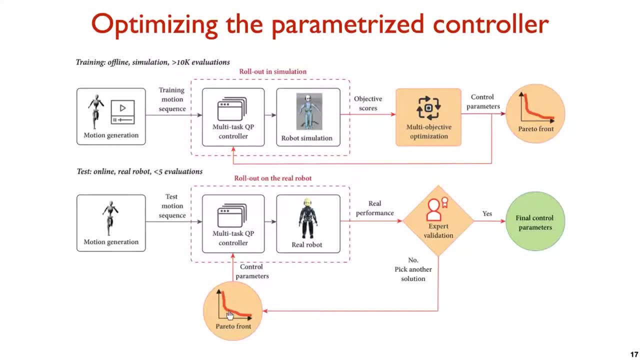 more human life. so we want to find a good set of parameters that are the trade-off between all this, uh, all these tasks that we, all the movement, just want to do. so our idea is to do a two-step parameter optimization. we have a first phase, that is, on offline, where we collect demonstration of 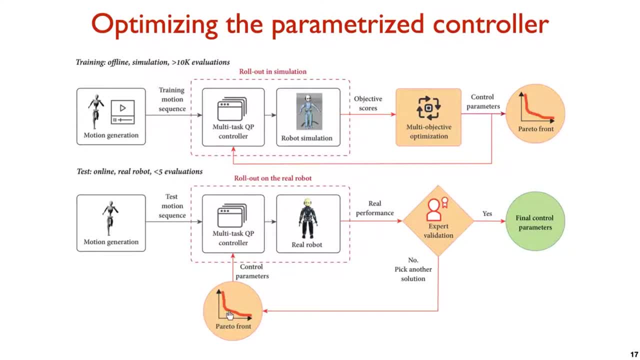 many different tasks from a human using the exam suit, uh. we inject them in our physics simulator: uh, with the uh, with many controllers. so basically, we play what the controller is doing with this, with this motion, and then we use a multi-objective optimization algorithm. we are using nsj2, which is 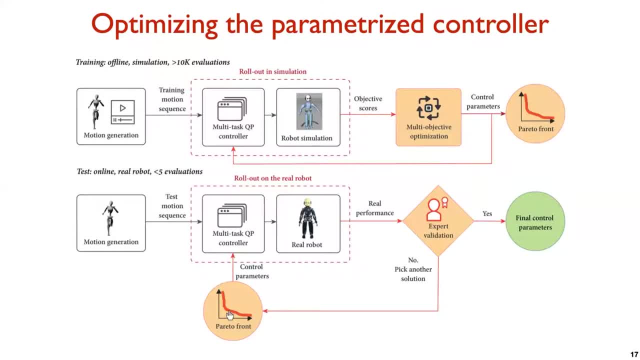 a pretty standard evolutionary multi-objective optimization algorithm to find pareto optimal solution. so at the end of this, of this big offline step, we end up with the pareto front and all the points in the pareto front are controllers that are validated in simulation on the simulated robot. then we have a second step, online on the robot, where we try. 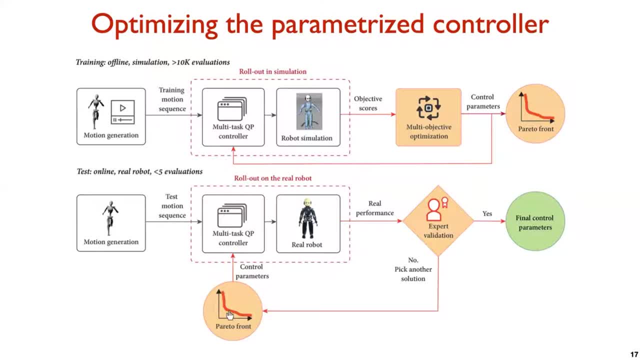 these points on the pareto front and then an expert decides if he's happy with the, with the behavior, with the performance of the controller on the robot. why multi-objective is because we don't have one objective alone, so we have many objectives and so we can promote solutions that are better in tracking the human gesture we can promote. 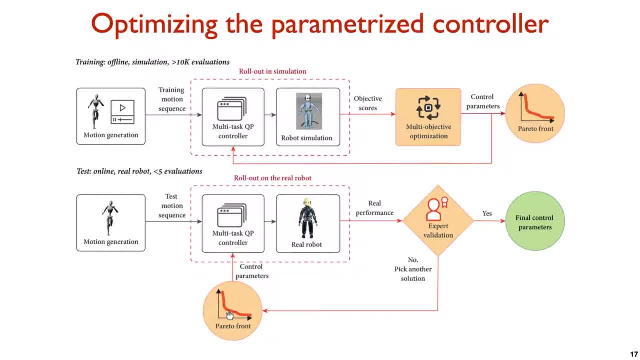 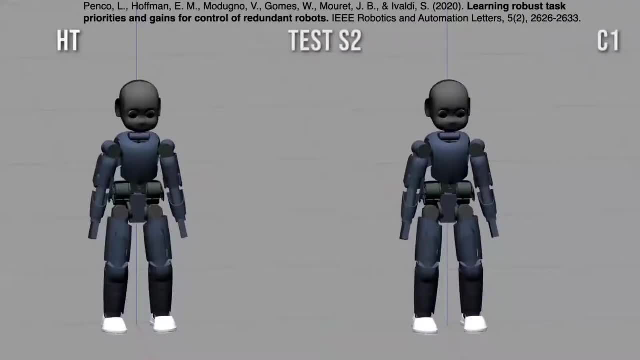 solutions that are more conservative. you know stability, and so maybe the robot doesn't fall if he has payload or disturbances. it's up to the expert, to this, the engineer, to the side. so, um, this is in. so it's important to reason like this, because, in in the case of icob expression, 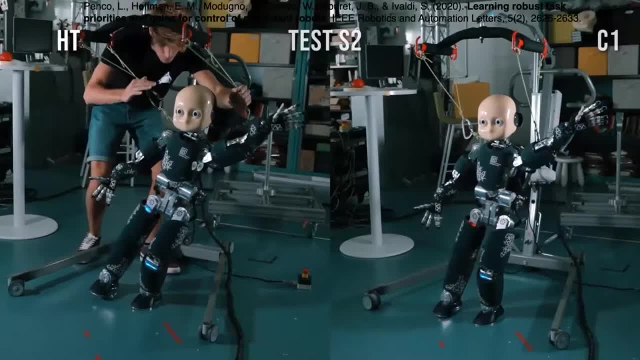 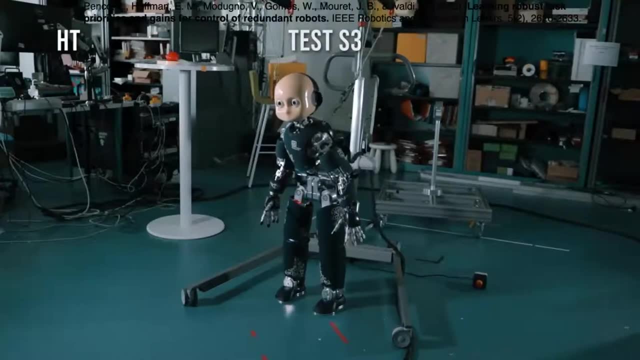 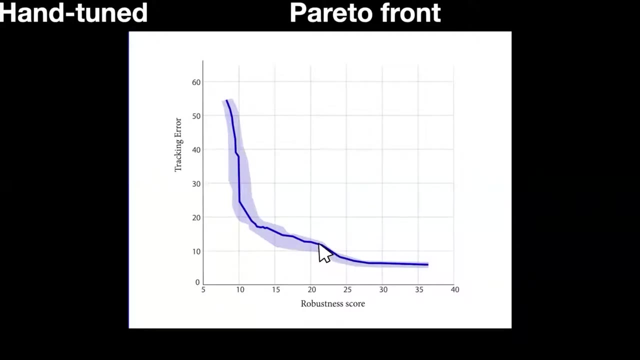 if you only optimize the solution in simulation, you end up frequently with solutions that are basically on the border of instability, um, and so a solution that works in simulation may not work on the robot, and so it's it's important that we that we have this, uh, double phase, and so the 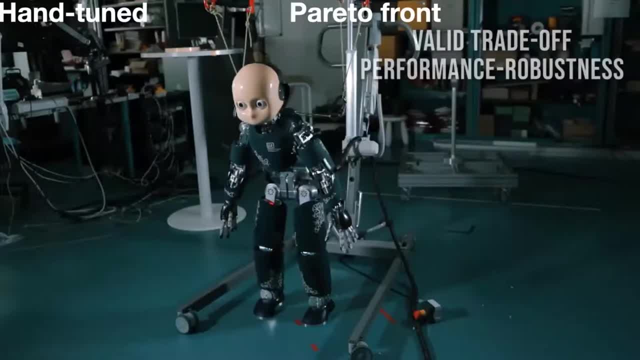 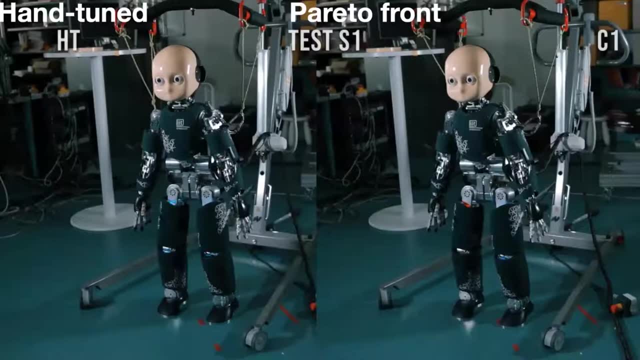 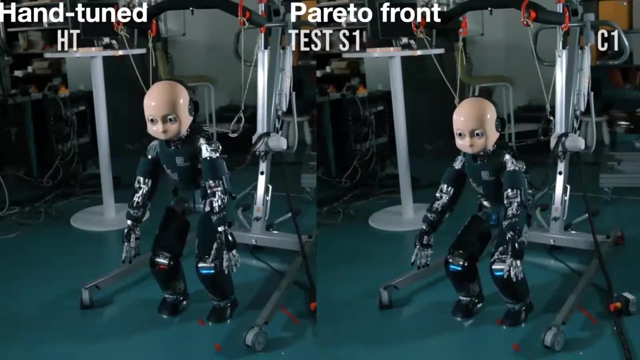 engineer can basically navigate the possible controllers in the pareto front and then it choose one and then it tries on the robot and usually with two, three trials we end up with a very satisfactory uh, and we tested usually. usually we tried with the motions that are very 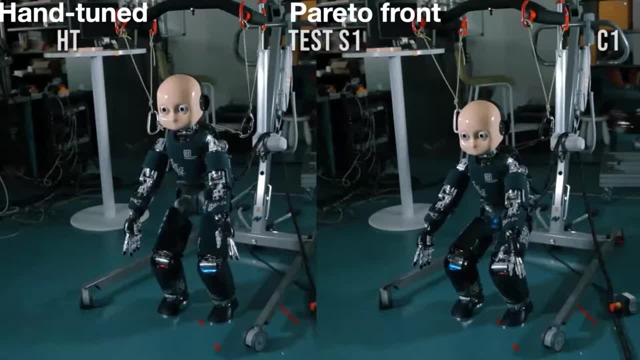 challenging, such as this squat. so maybe for human squatting is very easy, but for icab not. it's not easy because it's very challenging, for even its dynamic is very challenging, and so once we are acting, we have a controller. now we can use it for the operation. so here the robot is still operated. 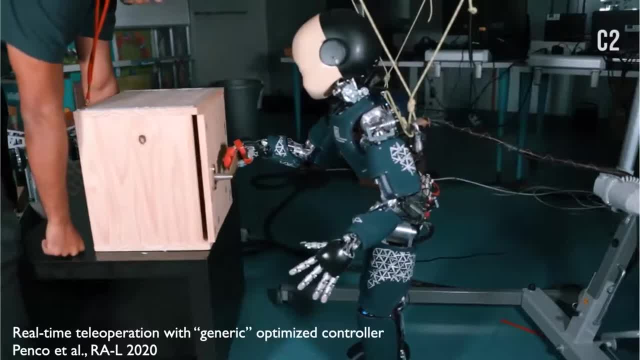 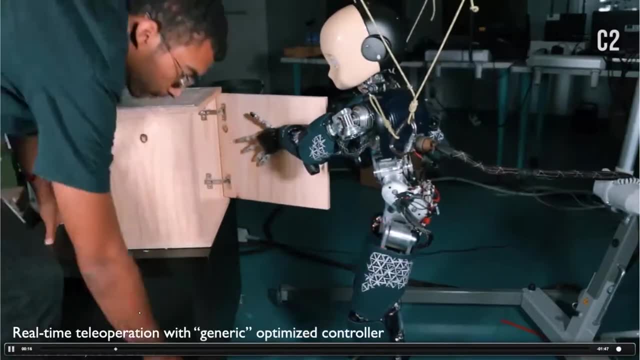 so there is a guy with the accent suit, and so the guy. so now this video is very long, so i'm gonna use my house to show you many different things that you can do. we are not switching controllers, so we don't have one controller for opening doors, one controller for picking, boxing or whatever it's. 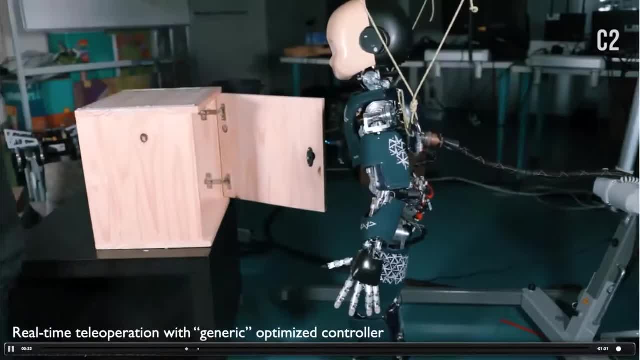 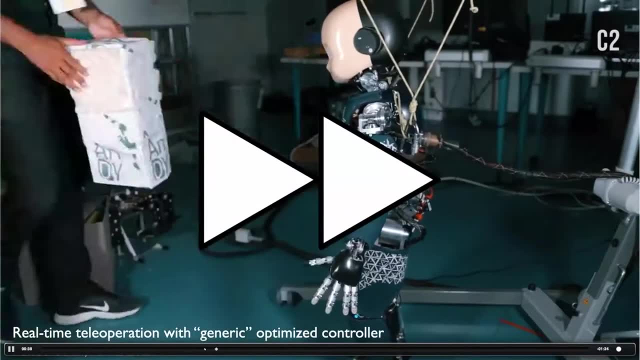 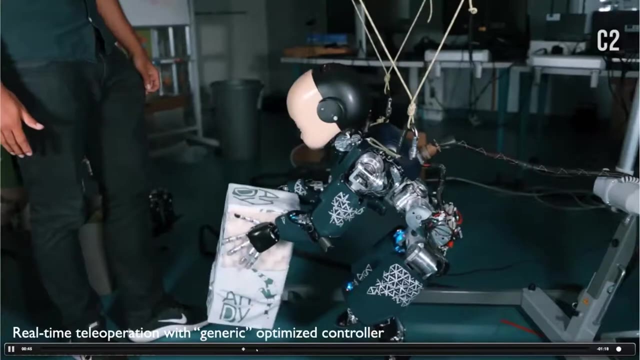 always the same controller and so the motion of the robot. it's not super fast, it's not somersaulting, but still it's acceptable to be a robot. and we are not. we don't have pauses, we don't have idle times. of course, sometimes it makes mistakes because for the operator it's difficult to know exactly how. 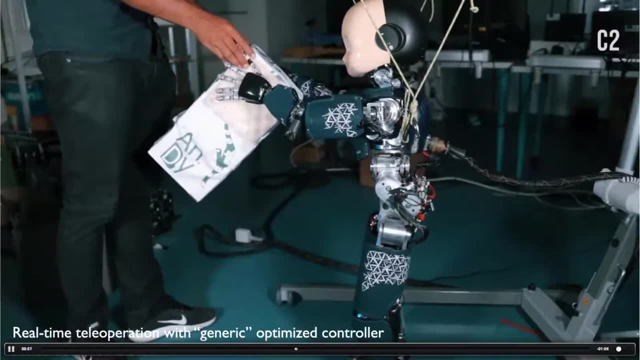 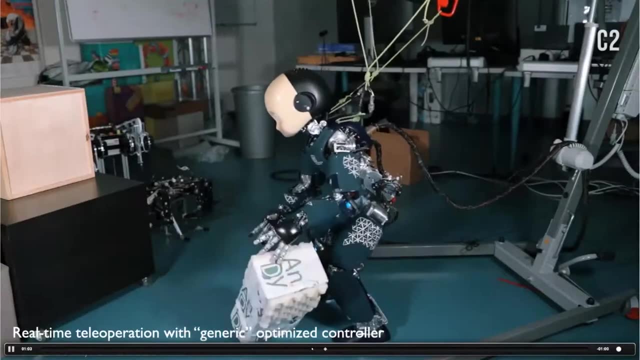 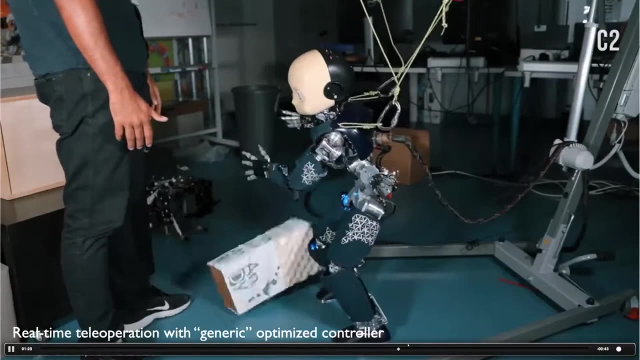 to interact with the, especially the environment, but still it works and you can see like it's picking stuff for the ground. this opening lacks. behavior on the archive is very dangerous, but it works and so we are happy. and then you can see the human is basically playing with the robot. 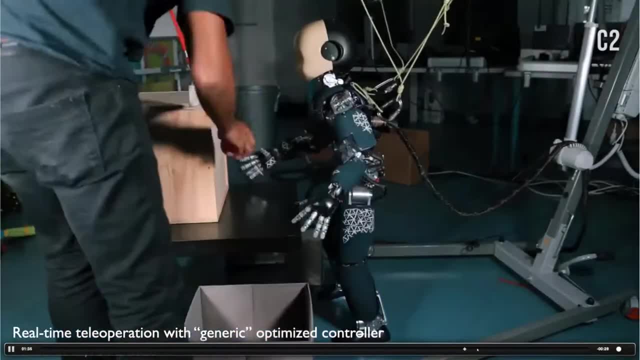 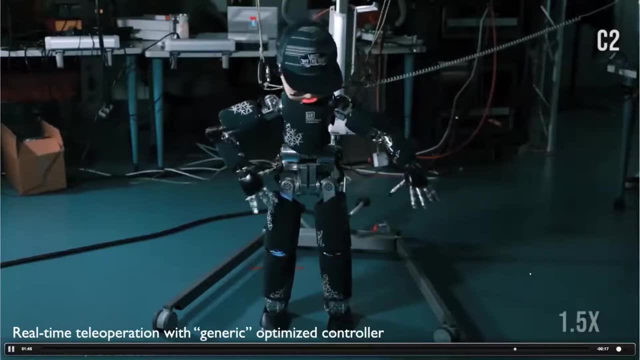 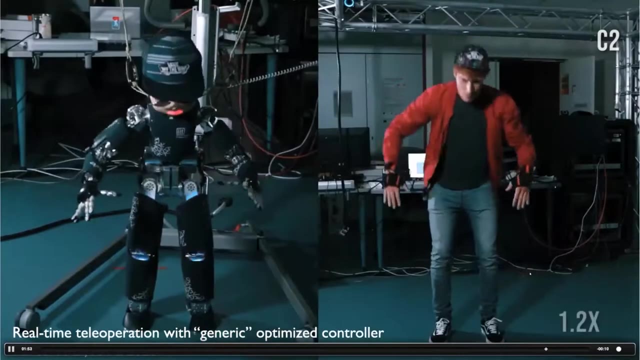 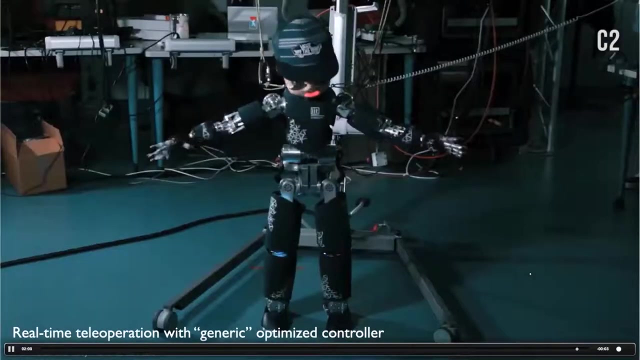 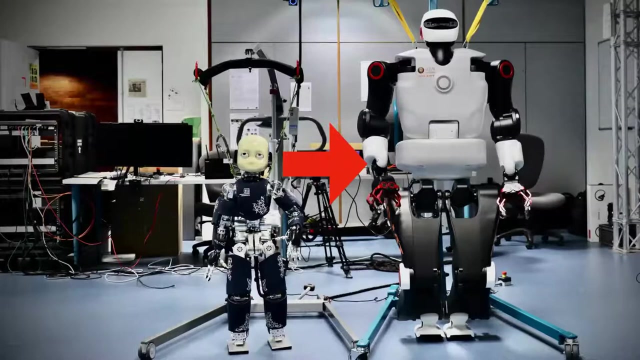 whatever, whatever you like, be creative. and then we also tried. so my student is very creative. he wants to paint his life in different ways to use this, and they can't do anything. so i'm so happy to be doing this, for them, to do something that they can't do, and they are very good at it, but the 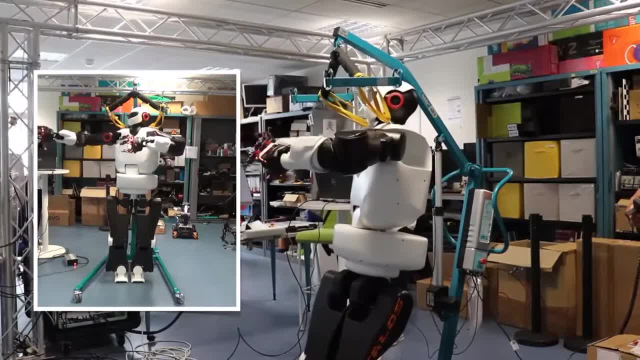 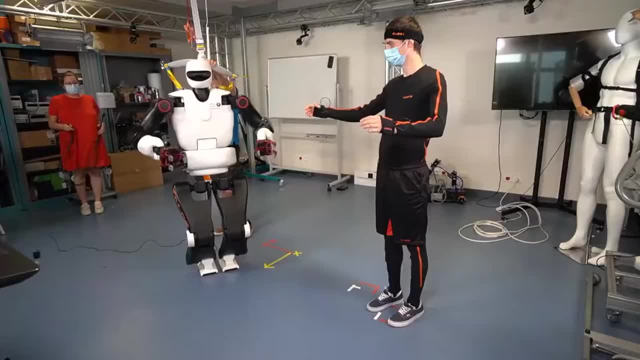 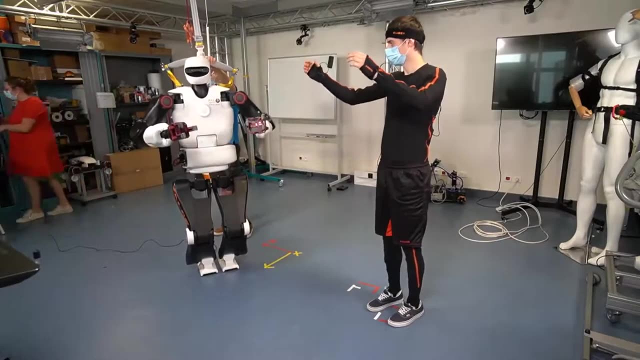 modifications. so here the talus is replicating the behavior that we're reporting on on the human. i don't have the audio, but it's very noisy and so we can do also the online targeting. so, as you can see, because of this hip structure of the talus, we cannot do. 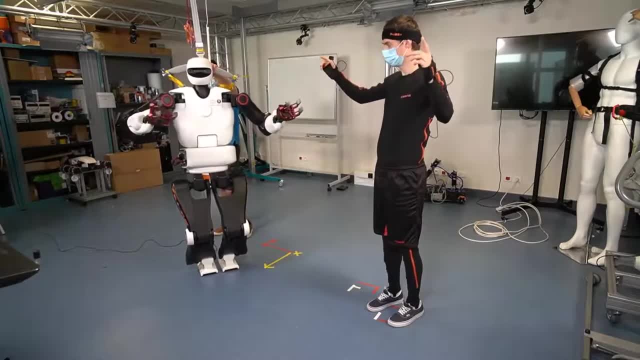 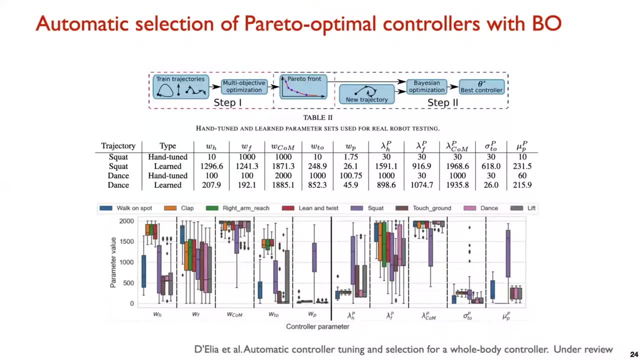 flexible movements, like in the eye cover, so it's less anthropomorphic. let's say: but see, let me. there are a couple of things that we can do with this robot. so we tried on the in the case of talos we tried to also to automatize completely also the. 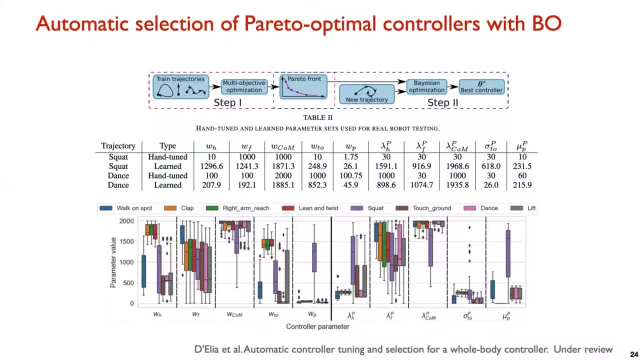 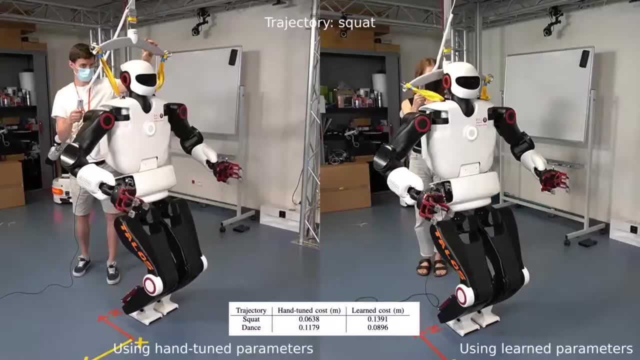 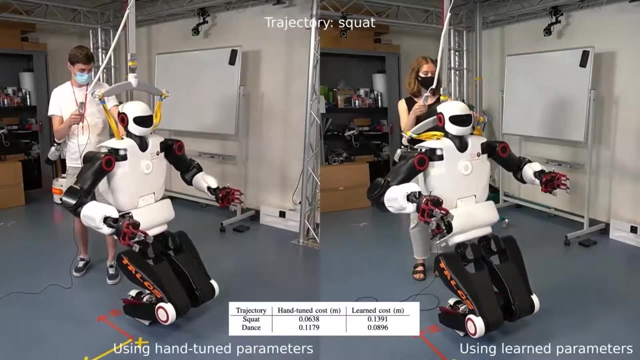 online tunic using base and optimization to look for the solution on the planet. of front, we didn't have a huge improvement, so we kind of abandoned this approach, even if it works, like in principle, so it can find its own controller on its own and- and we're very happy about this because, as you can see, like on on the left, you have a solution- 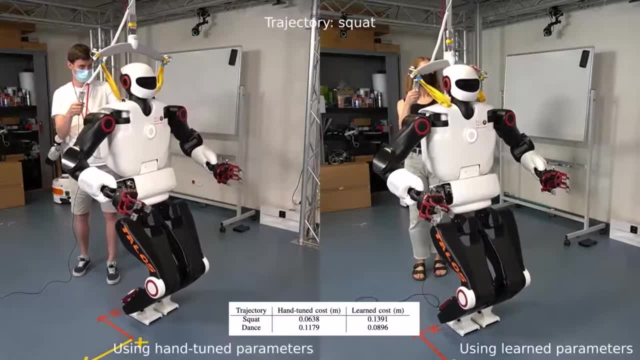 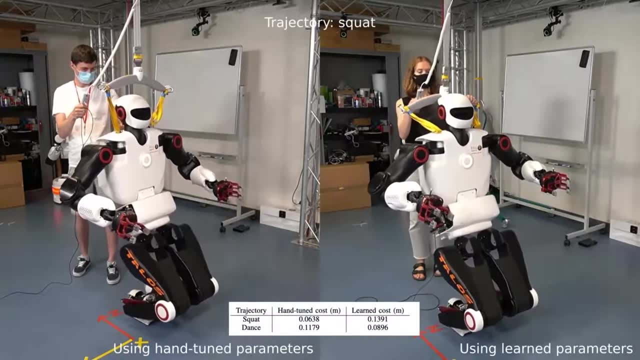 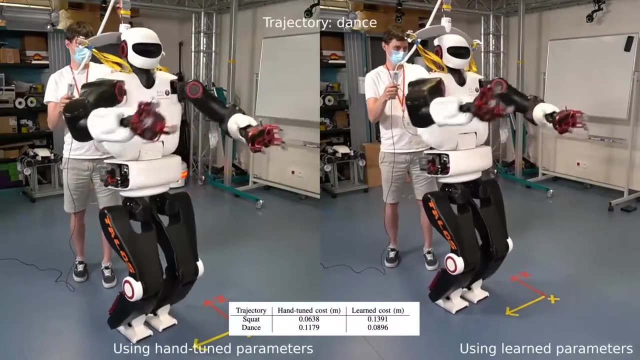 that was untuned by an engineer and, on the right, the solution that is optimal and, as you can see, the hands are are not moving in the arc while you do the whole body movement. so this is the kind of things that we want if we want to interact precisely with the, with objects, with the environment. 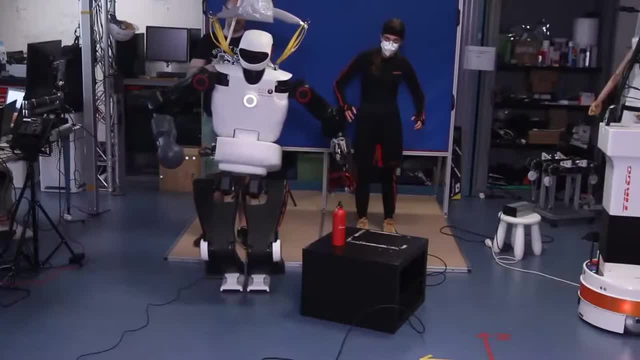 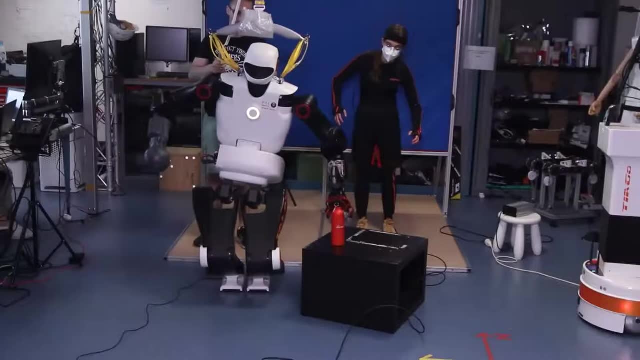 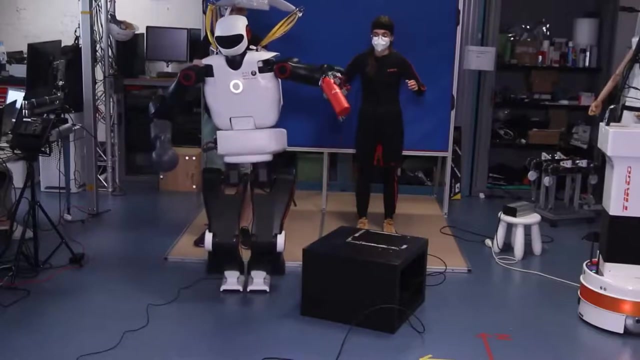 and so we can use it also for, like durum one compass stuff until operation. so the main problem in doing this right now is how to give the proper visual feedback to the operator- in the case of talos it is particularly difficult- and also to automatize the grasping with this kind of hand. 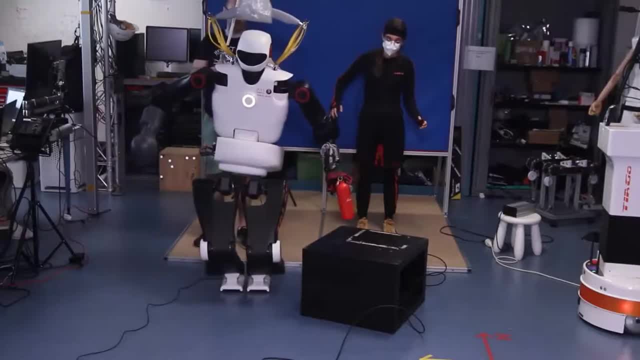 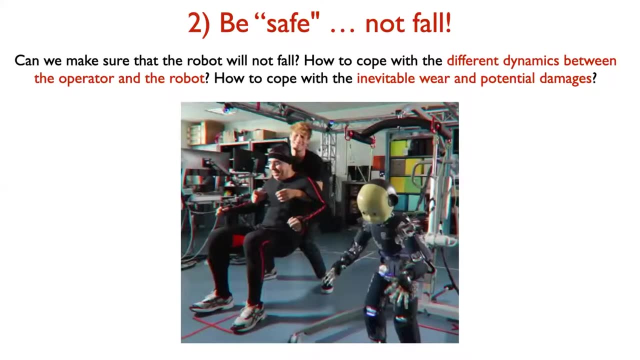 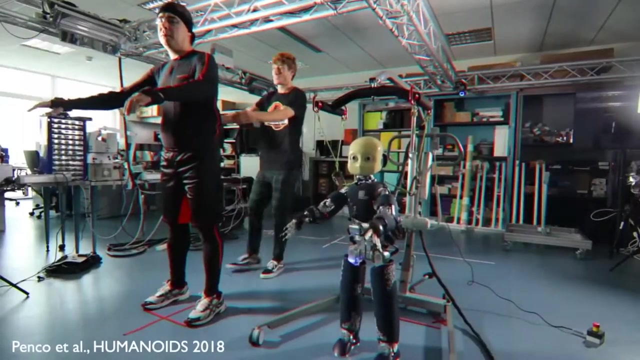 it's a good solution and, like, in the next month, probably, you will see more crazy stuff that we are thinking about doing. so the other problem that we have in this controller is about like being safe. safe is like just not falling. so a couple of years ago, uh, we, we showed that it was important, so this was the next exaggerated. 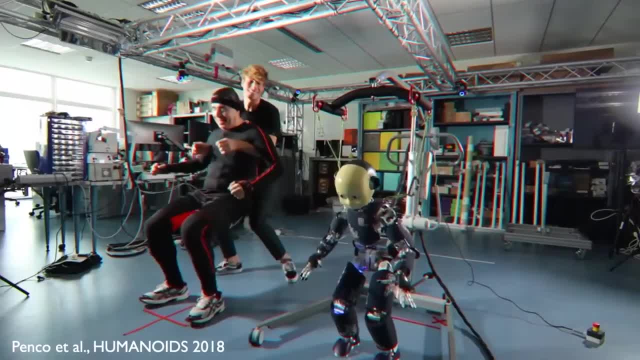 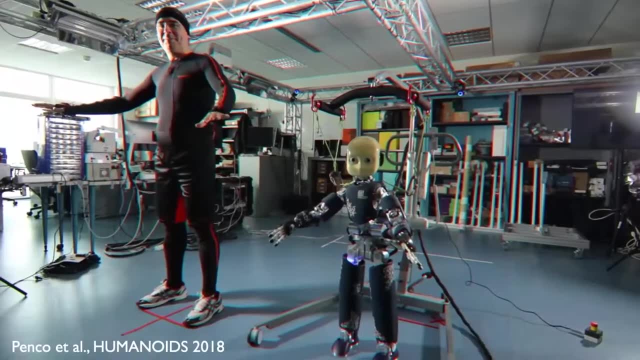 case like the operator is falling, and of course we don't want the robot to fall because we want to preserve the integrity of the robot. so this is a non-purpose exaggeration, but it was just to show that we were filtering the commands of the operator to avoid these things and 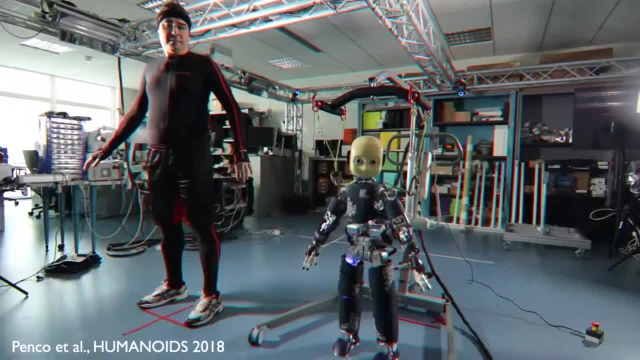 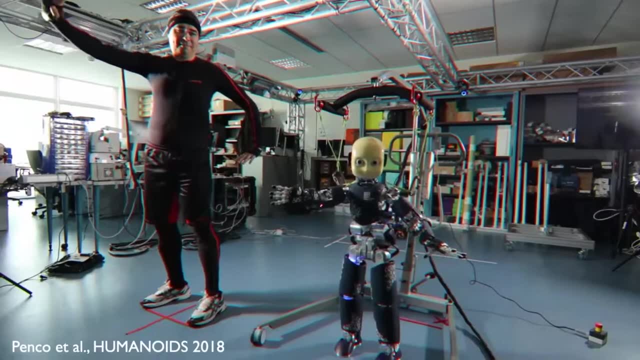 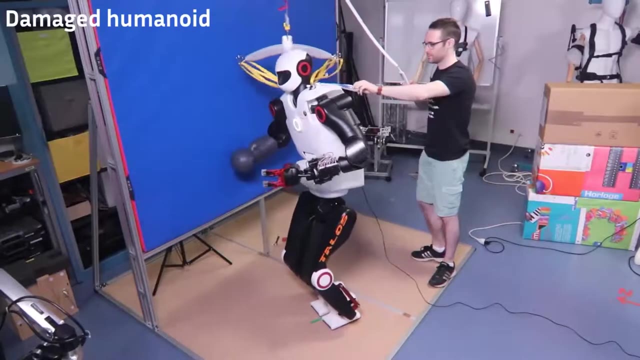 this guy here is a sociologist, so he's not a roboticist. he was a sociologist visiting the lab and he didn't know the work he was doing, so he didn't agreed him with the robot. but he he didn't what he said. he really didn't want to tell me the robot must have broken, so it wasn't that. 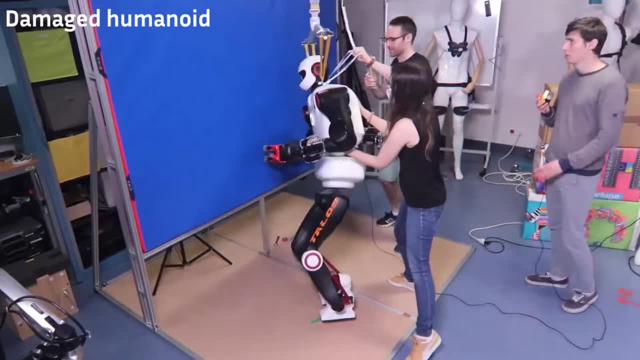 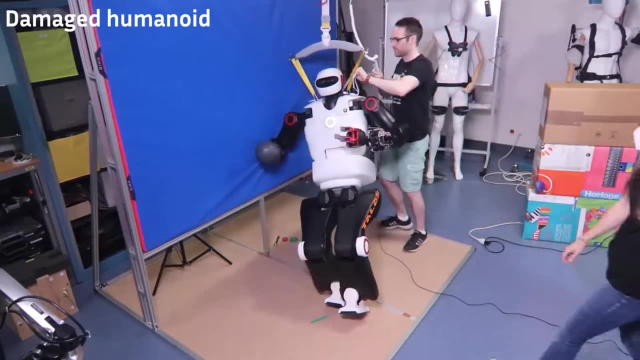 the robot is working. it just didn't work between humans and us. so when we think about in studies, what we see on the top right- is that the robot- somebody is taking a picture with robots. so the robot still works with humans, but it still works with people that are not roboticists. okay, this was a very simple 7p correction. so now we are looking into having behaviors that are resilient so that cope with damages. because imagine, if the robot is on the moon and it breaks, so it has to continue its mission, so it has to find a way to continue working even if it's damaged. 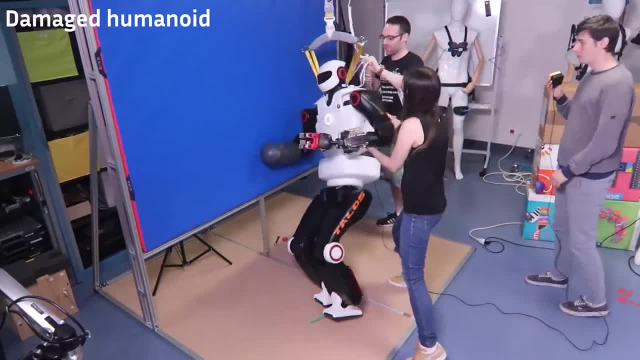 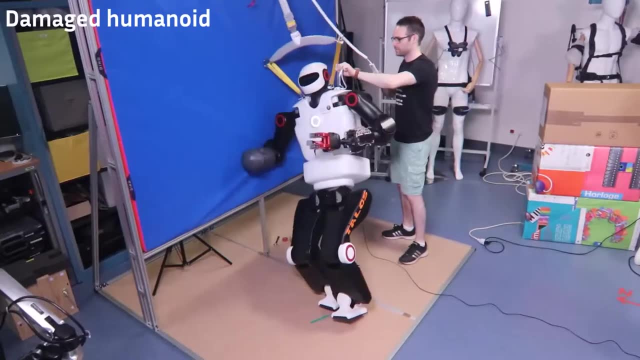 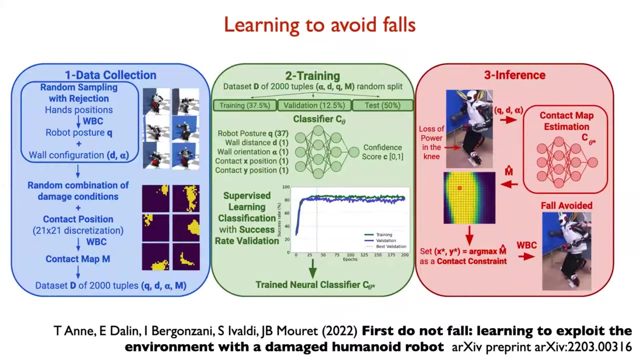 so here we are simulating the damage. we are shutting down completely the current on the robot one leg. so talus is 100 kilos, so if you remove entirely one leg it can fall, and so it makes a lot of noise like this. so what do we do to counter a damage? so we so this is a very recent work- that 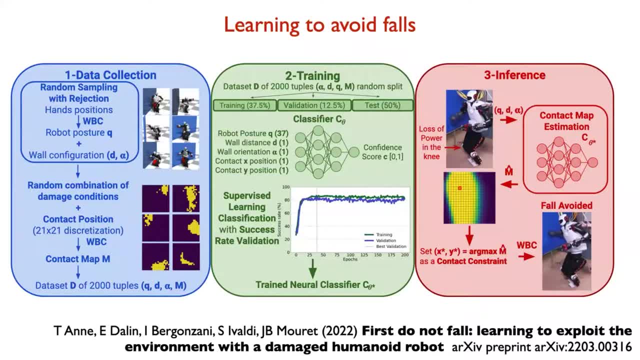 we did with timothée. so it's very simple. so we collect, we rely on simulation, so we simulate many cases of damages, many cases of the robot being in the environment. so the only position hypothesis that we do here is that the robot knows that there is a wall, otherwise generating for a variety of 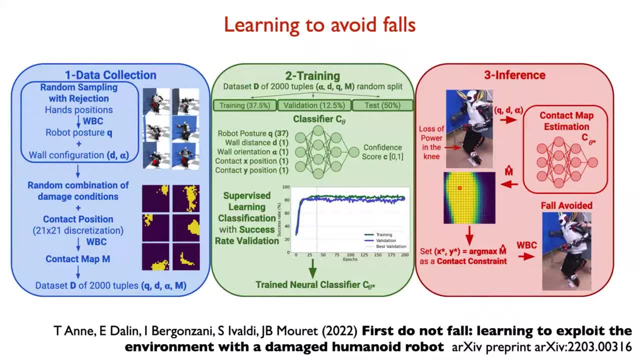 environment would be very difficult, but in principle it can work with other environments. so here we know that there is a wall. the robot tries, generates a diversity of behaviors- to lean on the wall, so it's looking for the position where to put the end in a reactive way so that it can. 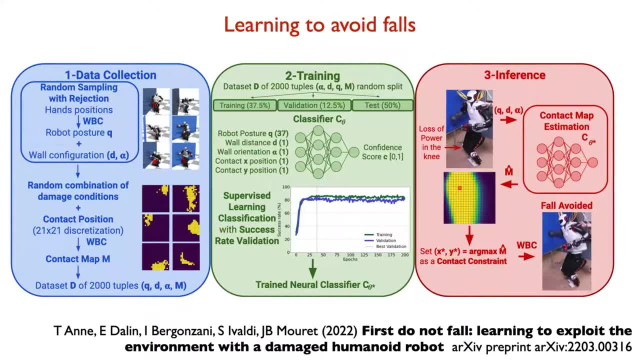 lean on the wall and so we basically learn- than a classifier that we can use to predict in which location we can put the end, given the current posture of the robot and the current uh wall situation, so that we can generate adaptive behavior immediately in case of a damage, to avoid falling. 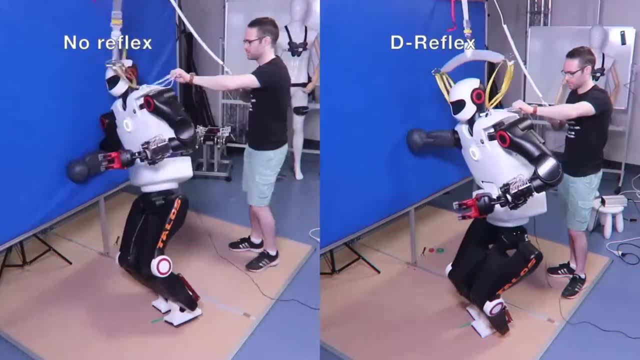 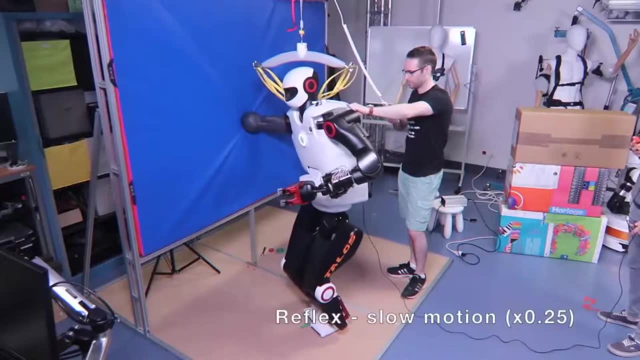 and so this is what happens. so in on the left is without the this reflex mechanism and this is, and on the right with this reflex. so this is in slow motion, it's very, very fast and because if we were not faster the robot would fall, so it would be catastrophic. 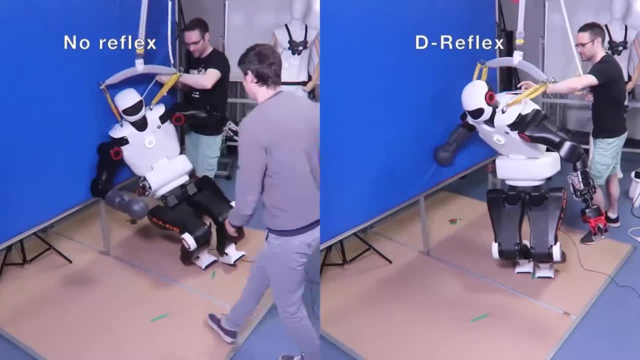 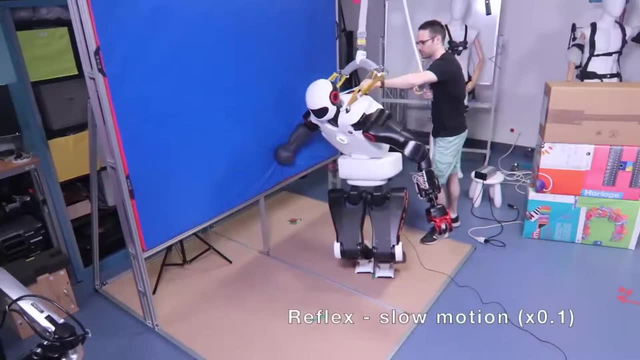 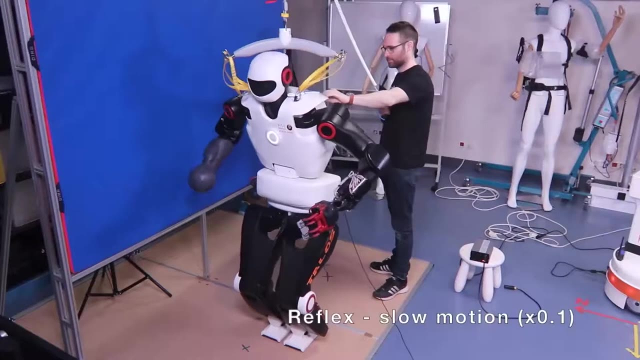 so basically, in that moment when we have a damage, we switch to a simpler controller that is not tracking the operator or doing the task that he wants to do, it's just a safety controller that is like quickly reacting so it doesn't fall. and here it's again. we are shutting down, so there is no. 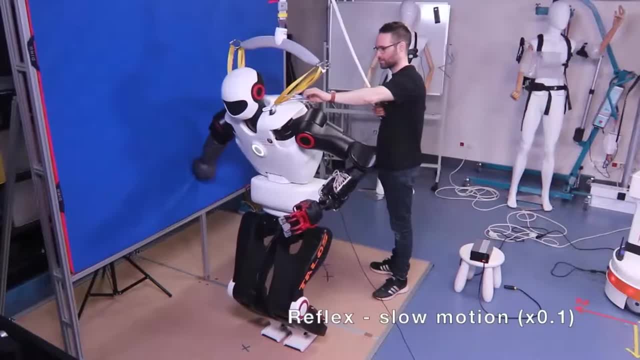 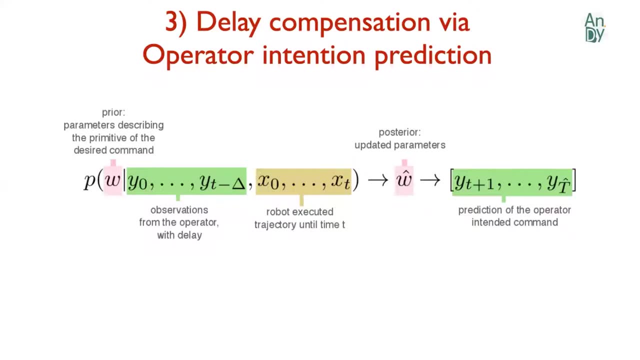 current on the right leg. so the last problem we want we are working on is delay compensation because, as i said for the operator is with the smallest delay there is a huge problem, like you don't know how to do, what to do really on the robot, and if you are doing gestures in the air it's not a big problem. 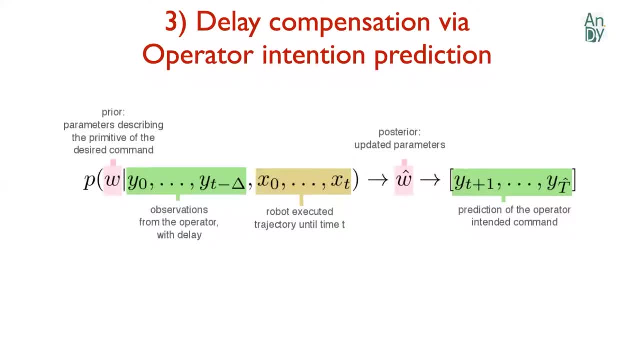 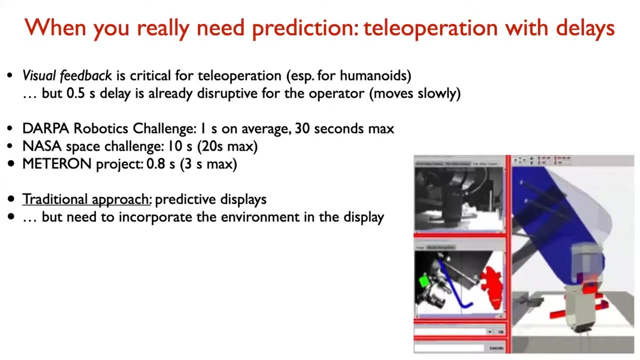 but if you are trying to manipulate, open a door or picking something with precision, this is catastrophic because the operator doesn't know if he's doing it correctly and so on. so there are many cases actually where so current projects, where they are working on teleoperation, with delays. so you all know that our robotics challenge- the connection was that- was delayed. 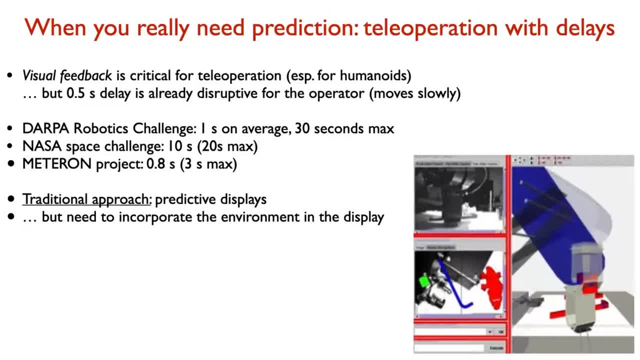 and then there were a lot of perturbation. same for the nasa space challenge metron project, i know. if you are aware, it's robots that are on the lr and they are teleoperated from the iss by the astronauts and there is like the delay from iss to the earth and, for example, in their case they use the. 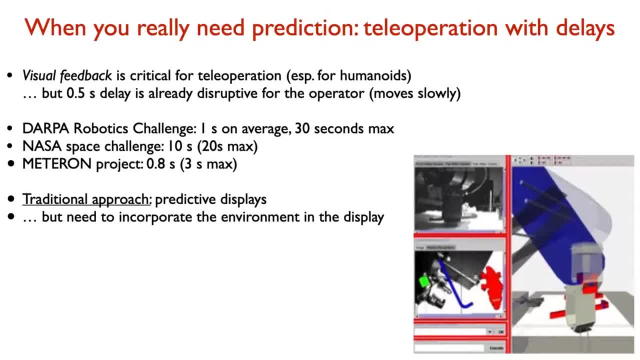 approach of having predictive displays. so they have a display where you have a digital queen of the robot and of the environment in which the robot is acting and you show basically the future. and if you read, like the papers, that they do, that they write, they say that the astronauts after a 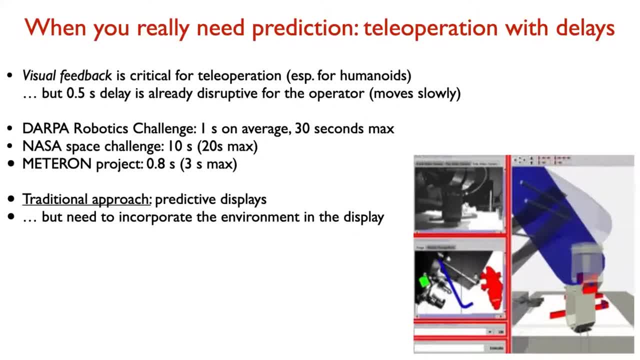 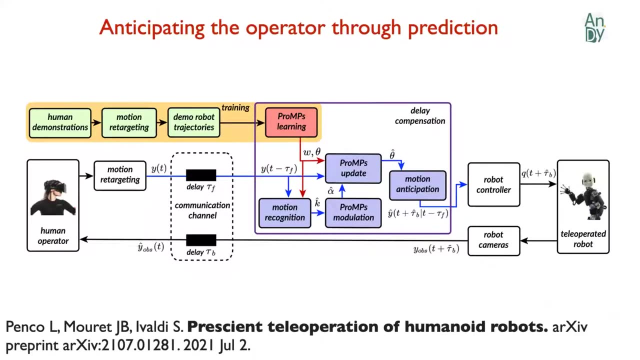 certain uh delay, they are completely like crazy. they have a vomit and motion sickness and it's very, very also cognitively it's very, very difficult. so we decided to have another approach. so we are anticipating basically the robot, so we make a prediction of what the robot is going to do. 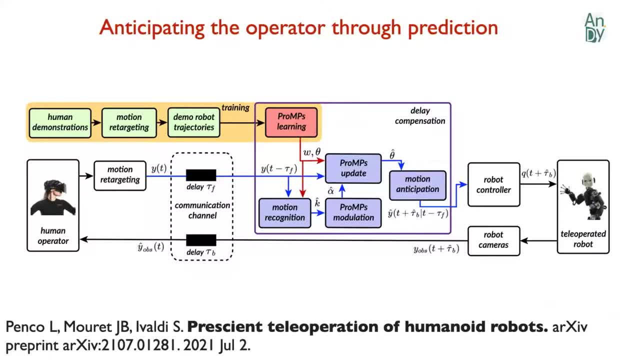 and then the robot is executing the motion before the operator is weird. so to do this, uh, we rely on uh models of uh of the movements that the human, that the human is going to do on the robot, and we learn these models using motion primitives. this is a 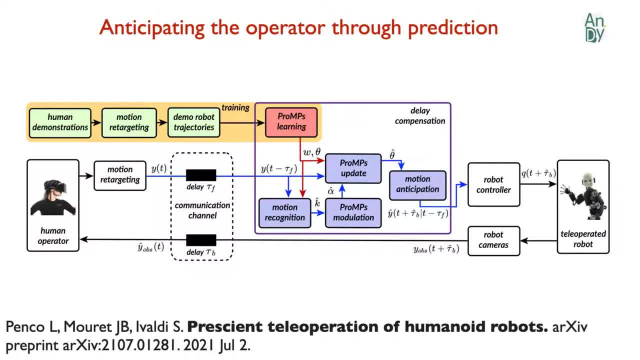 very standard machine learning techniques right now to learn motion primitives, manipulation and so on. so in the past we have used a lot from this emotion primitives, which i will explain in the next slide. they are work very well, they're easy to use and what we do is that basically, um, we take the prediction of the future of seconds of movement that the operator is. 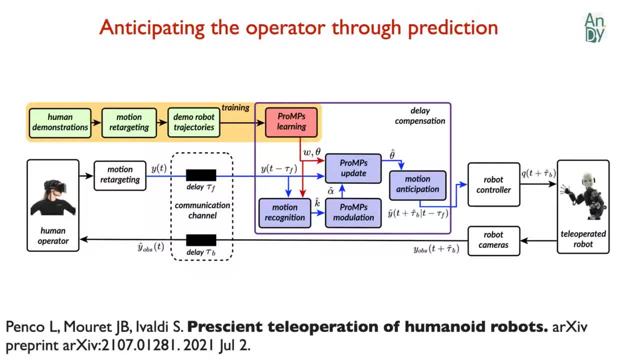 going to do and we let the robot execute this uh prediction and then we have a little uh sharp control loop correct so that the prediction that matches what the what the operator is actually doing. and this is the only feedback that we have here is visual feedback, which is: 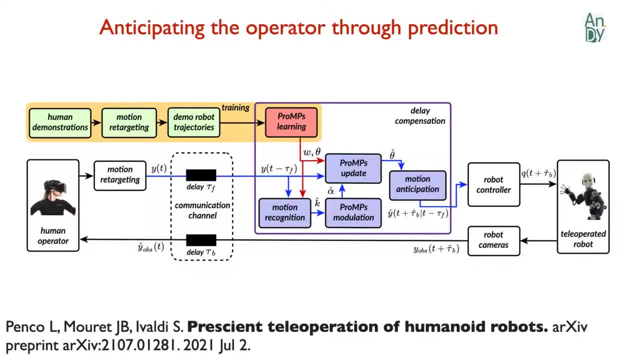 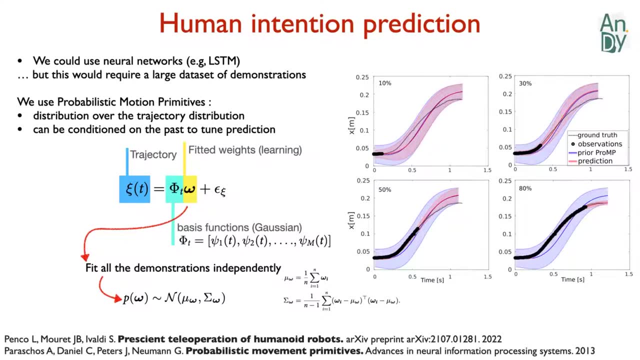 this technique is nice because it allows to have a visual feedback that is aligned with what the human would do if there was no delay. so this works with the, with the prediction, with the motion primitives. so motion primitives are basically a variant of gaussian processes and they allow to learn a probabilistic distribution. 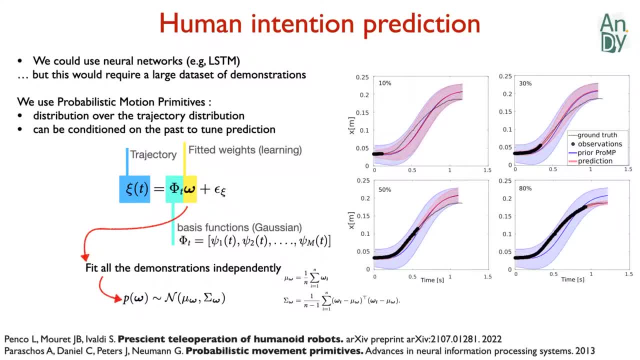 of a demonstrated trajectories so you can learn the mean of the demonstration of the of the primitives, but also like the variance and you can use it for what you want to do. but the nice feature is that if you have a model that is learned and you have observation of an ongoing movement, you 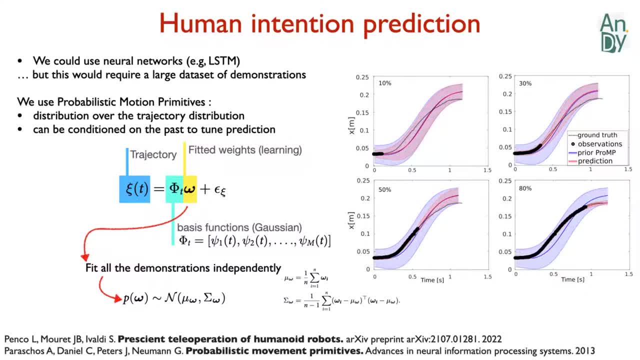 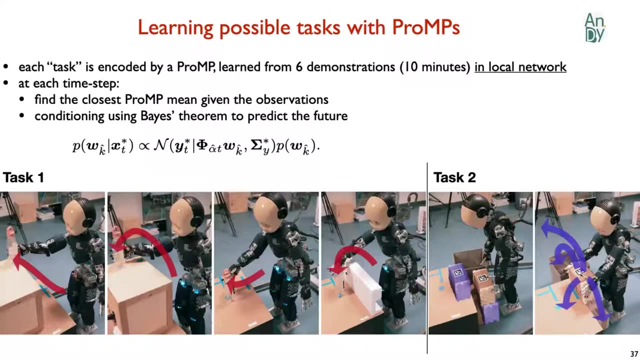 can use this observation to condition the distribution of the of the primitive and to make a complete estimation, so the prediction of the, of the follow-up trajectory, and this is exactly the property that we are using, exploiting. so, if the robot has to do many different movements for every type of movement, 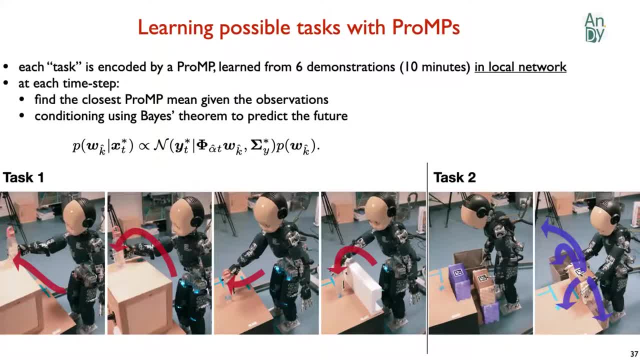 we learn a primitive and the primitive can have some violence. for example, they can incorporate presence or not of obstacles, the the final object can be moved to a different location and so on. and this is very important with respect to the classical manipulation grasping scenario we are. 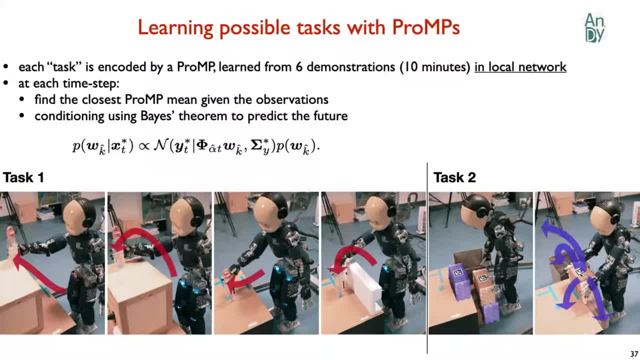 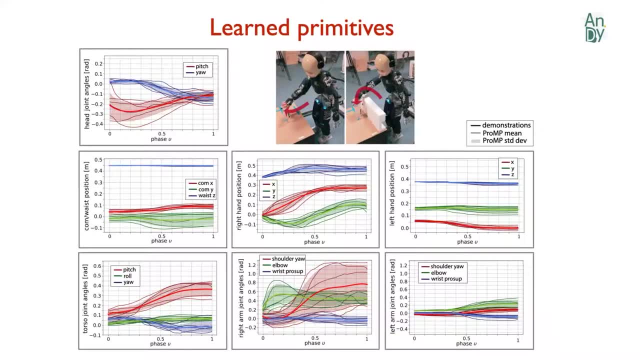 not only learning the primitive of the arm, but the primitive of the whole body, the entire body, because the entire body is moving. so if, for example, for this kind of simple experiment where you're picking an object, you're not just picking an object with the arm, you're picking it with the entire body. so if the object is on the ground, you have to, you know, go on. 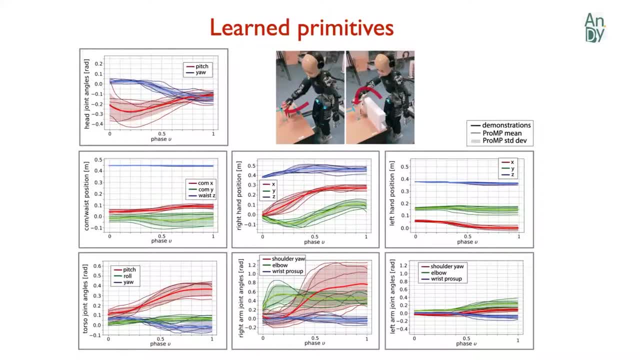 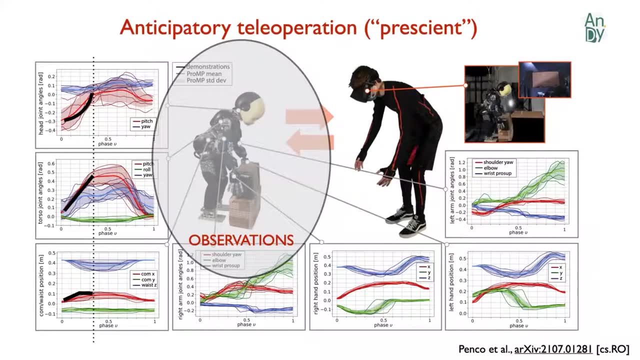 the ground as well, lower your center of mass, and so we have limitations for all the trajectories for the controller. so and then, when we have all these primitives, during thefront operation, we take the observations that come from the retarding force. during the teleoperation, we take the observations that come from the retarding force. 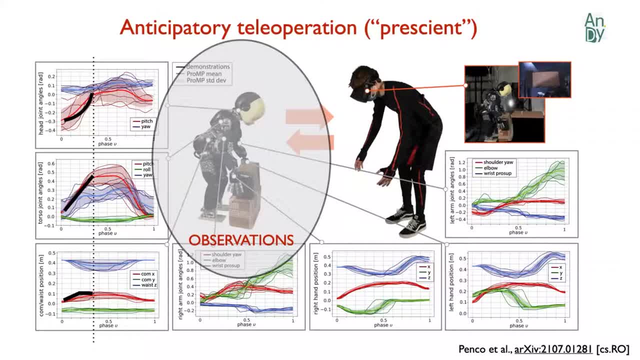 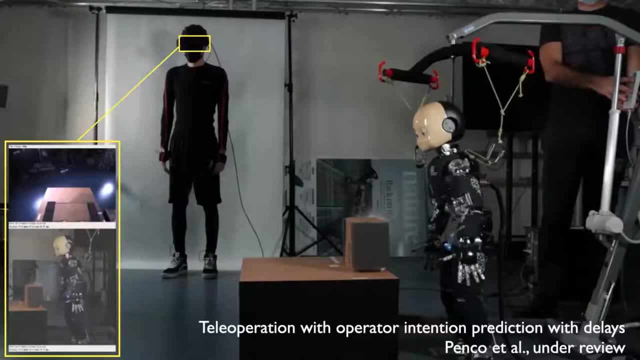 targeting of the operator and then we condition, we predict what the robot should do in the next seconds. so now it's a bit difficult to see because the robot is going to execute the command of the operator before the operator is doing it. so you have to look at. now i will have boxes to show you. 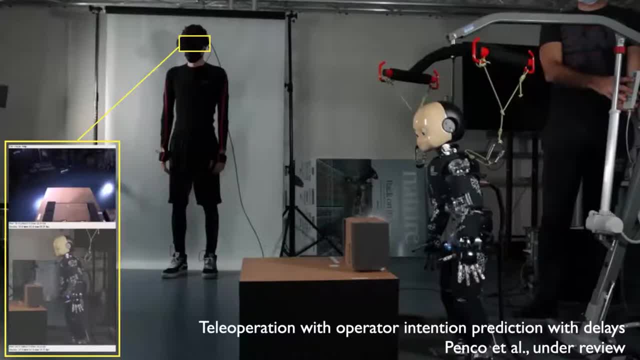 what to look. so this is the box where you see the visual feedback of the operator. so you have, on the top you have the visual feedback from the, from the cameras of the robot, okay, and on the bottom it's an environmental camera. why did we have this? because otherwise it's very difficult, very, very. 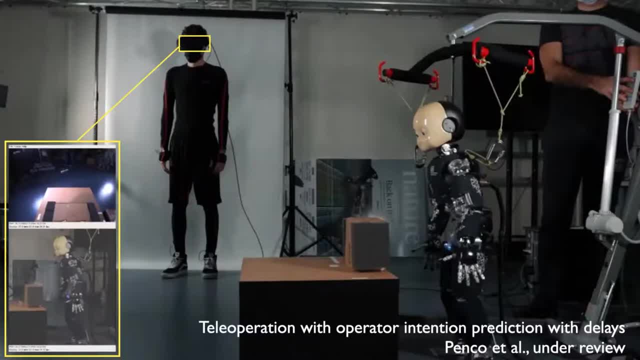 difficult for the operator to pick objects in a reliable way, so we need more environmental awareness. environment awareness- okay, so this is the first thing to watch. so when, when you will see the operator moving, try to look so he will move the head first, so you can look at the head first. 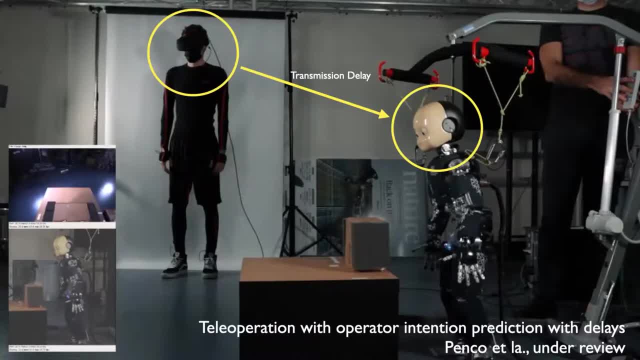 there was be a transmission delay. so now this is the experiment of 1.5 seconds. i chose it because it's the one of the most visible. so there is a 1.5 delay from the comment of the operator to the robot. so we are inducing this delay artificially, so when the human is moving the ad, then the robot 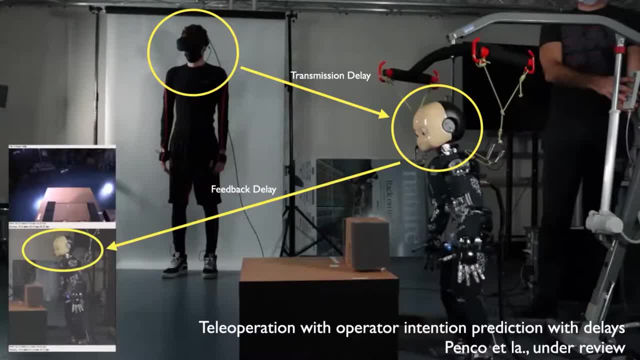 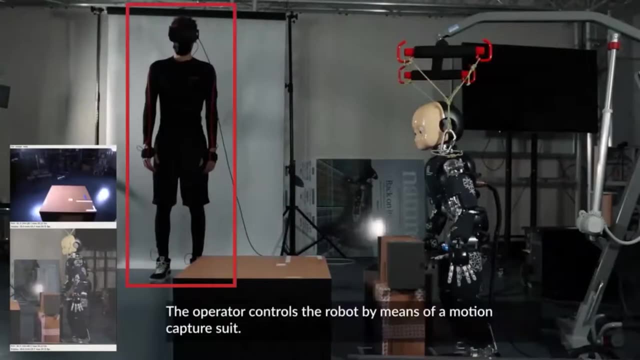 will move the head after 1.5 seconds and then the feedback will appear to the robot, to the human, after 1.5 delay. okay, so the visual feedback will be delayed as well because the, the, the delay is in back and forth. okay, so you see this. so the operator controls the robot with. 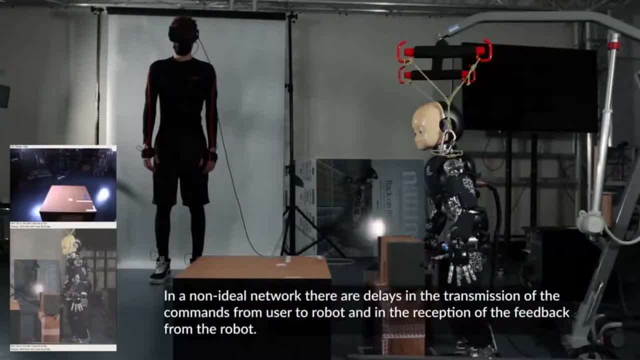 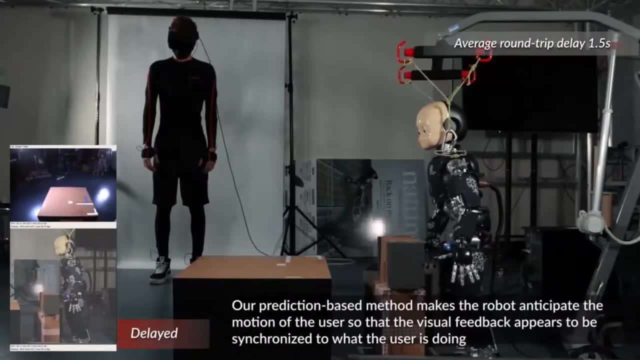 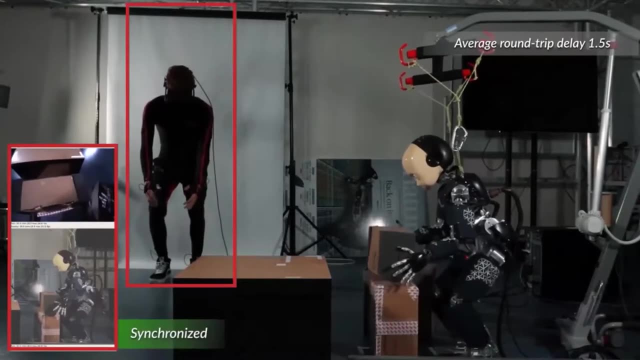 the suit. this is the visual feedback. in the non-ideal network, everything goes well, it's immediate, and then you will see that when the human is moving- so now it's moving- the robot is moving- the delay there is synchronizing. it means there is computing, the prediction and now the robot is doing the task before the human is doing it. 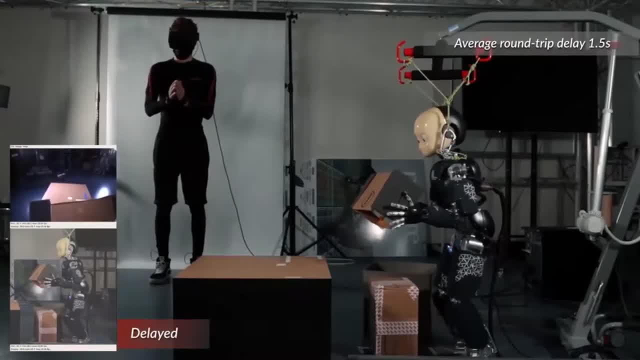 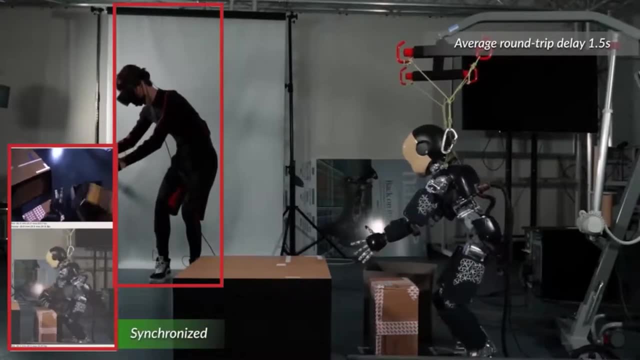 and the human has the impression that his action from the visual feedback are synchronized with the one of the robot, but the robot has already finished the task. and then, of course, this is a prediction that is based on primitive. so every time that you switch the behavior to switch the 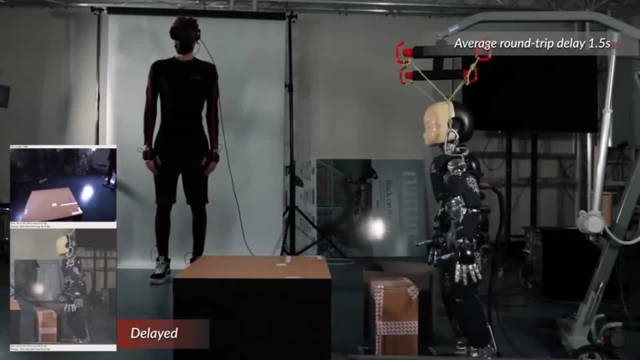 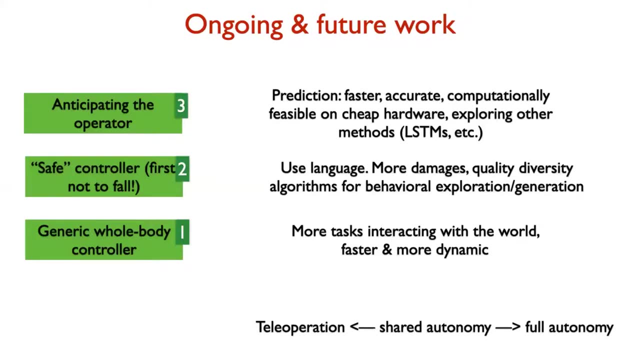 task. there is a new primitive that has to be predicted, which is something that we want to get rid of, but it will be for later, okay. so to sum up, we saw three problems that we have with the human operation, generical body controllers. so in the next future, like ongoing. next, we want to add more tasks. 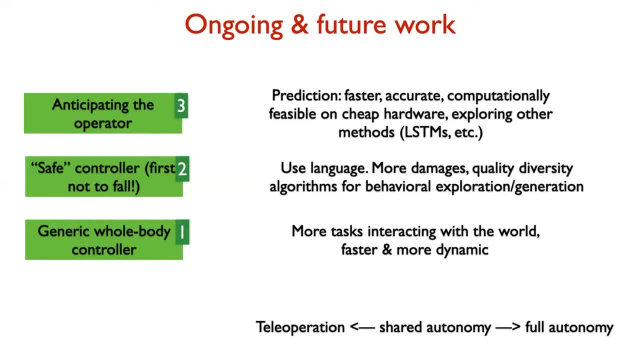 especially. we have a challenge now where we have to do a variety of tasks where the robots interact in a household environment, so we will have more things. we want to go also faster, because the operator is still moving very slowly. upgrade, let's say, the safety part. we want to use language on one side. 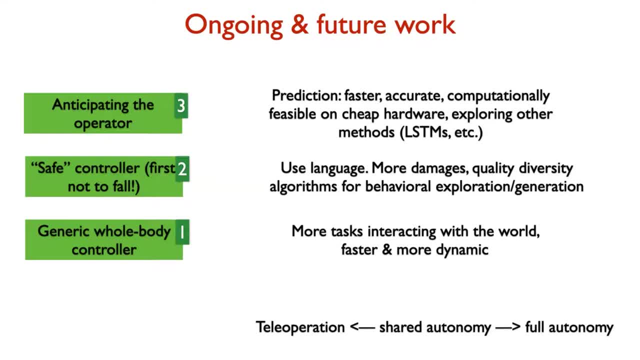 there were many tools during this conference about using language, so there is possible improvement that we want to add. and then, of course, explore more damages, and we want to also add quality diversity to explore more range of behaviors that the human can do. and then, for the third, 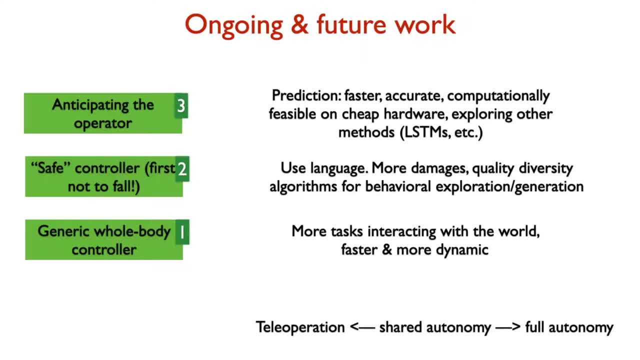 part to have better prediction, faster, more accurate, but also computationally feasible on board, on the computer of the robot. and so, to let you know, we are using this technology on humanoids, where we are also exporting in our active exoskeletons that have not a lot of. 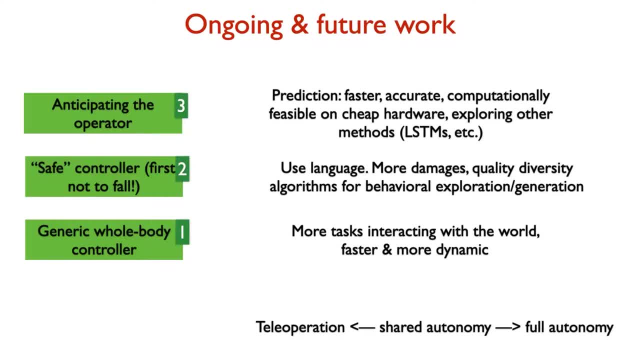 capabilities. um, so we want to be faster, and you know, computationally. and then, even if we like collaboration at some point, to with that the robot to say, hey, i know how to do this task, i can do it on my own. okay, so i can do it autonomously. so that's sometimes the end, what you're already a behavior. 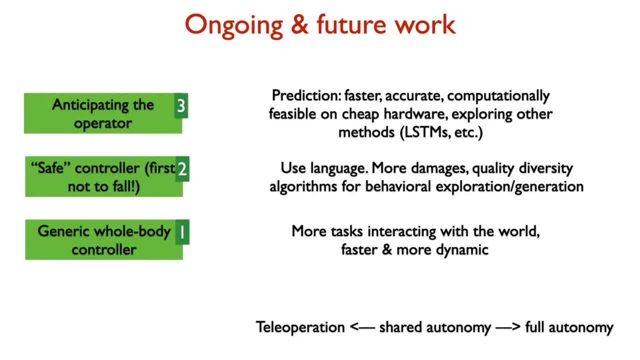 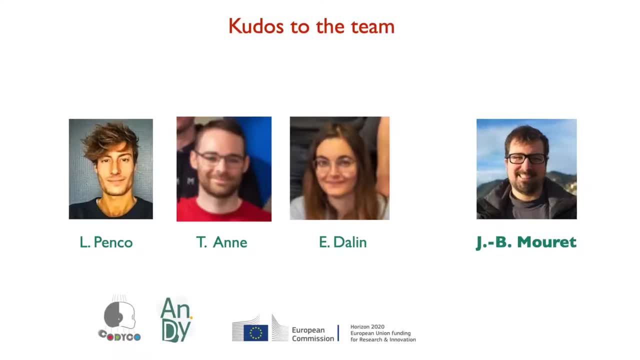 So we will use the transition from teleoperation to autonomous And the CTS is the people that work with me on this project and, in particular, Jean-Baptiste Moretti is a colleague And we are hiring because we have a European project. so if you want to do a PhD or a post-doc, 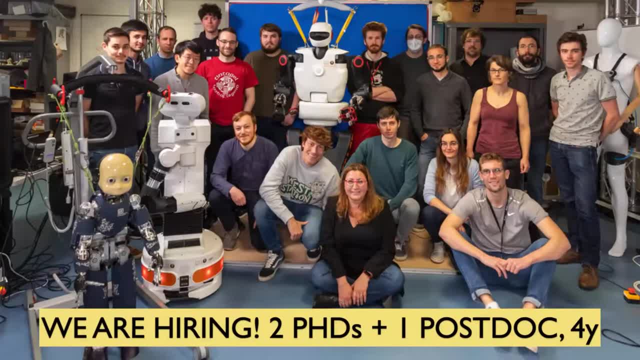 let me know. So thank you so much for your time. Are there any questions from the audience? Yes, It's your prediction on the teleoperation. Did you go into a task that you did not during training, or was it a mental craze, or is it? 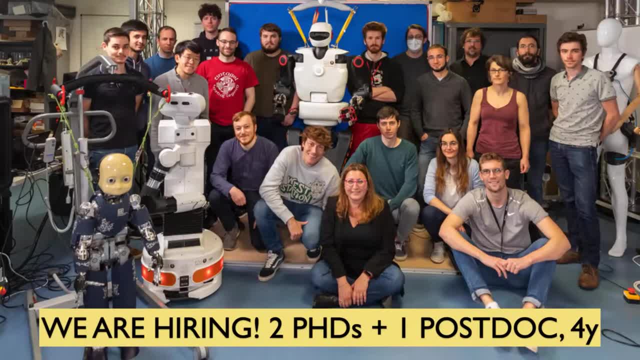 reliable? No, So if you use motion primitives, these are really supposed to be so- the tasks that we can execute and predict for are supposed to be belonging to these motion primitives. So actually, if you have, imagine you have 10 motion primitives and you do one action, 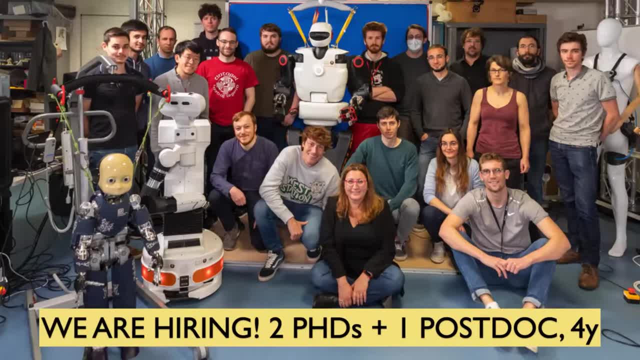 you don't know to which primitive you belong. So you have to compute a likelihood to figure out which is the primitive. And if you don't, then you will not have a very reliable prediction Because you will make a mix. You can use a mixer of primitives. 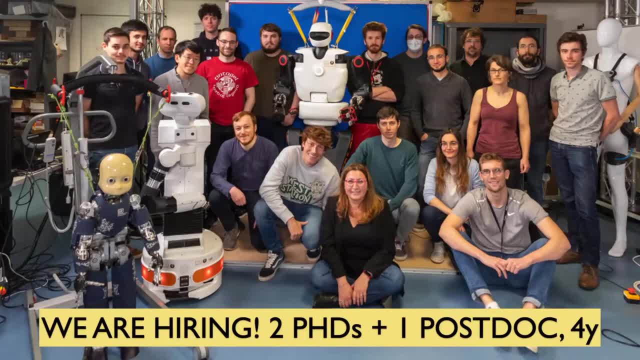 Actually, there is a nice feature of these primitives: it can blend them, so you can have a prediction that is a blending of the prediction of all the primitives that you already know. But to address your point, actually we are looking into just a neural network, that is. 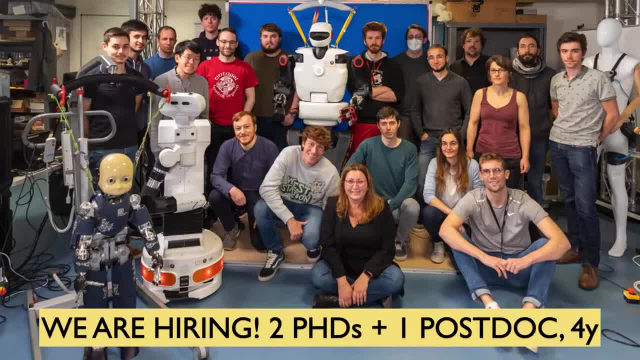 agnostic of the task that we are currently doing, because this technique with primitives- the next feature- is very easy to divide. to divide, This is only for the predictions, only for the prediction, because we wanted to start with something that we know that is very reliable in prediction. but we are doing it also with 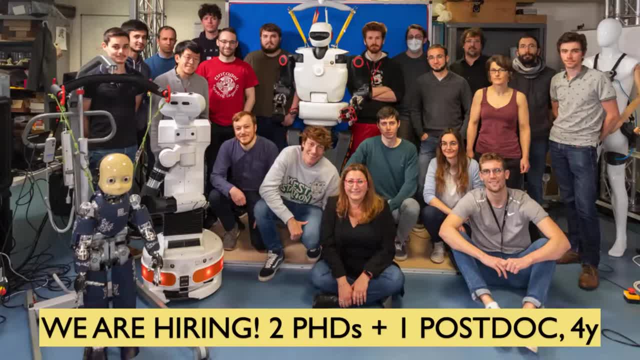 the neural networks that don't have really a knowledge about the task that you're doing. So we have one question from the chat, excuse me. Yes, Have you observed a singularity issue during human-robot motion mapping? Can you repeat it for the people that are not? 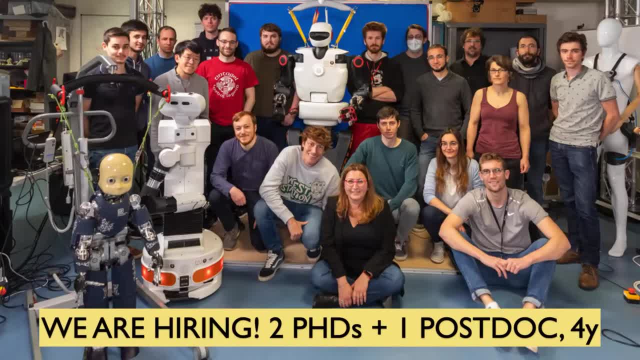 Yes. One question: Have you observed a singularity issue during human-robot motion mapping? I don't know what is the singularity issue. No, this is solved by the whole-body controller, so we don't take care about that. there is.